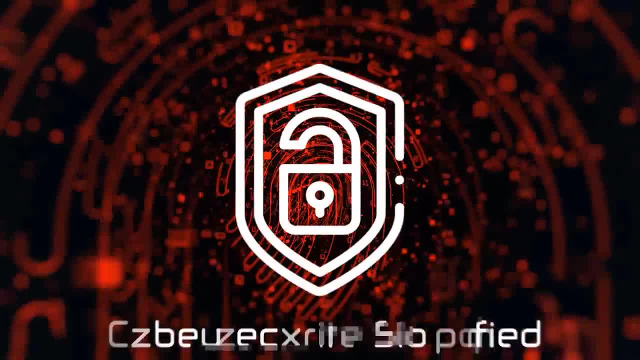 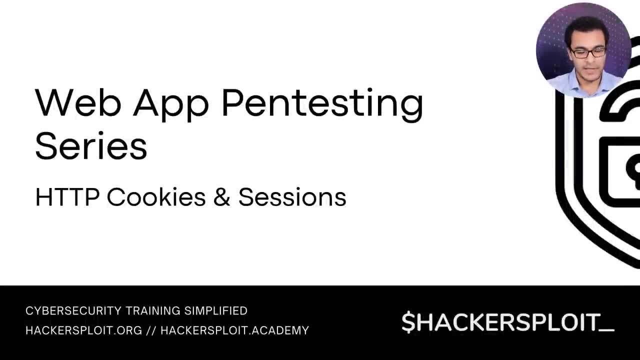 Hey guys, Hackersploit here back again with another video. Welcome back to the web app pen testing series. In this video, we're going to be taking a look at HTTP cookies and sessions, So this is arguably one of the most important videos in this series, primarily because cookies. 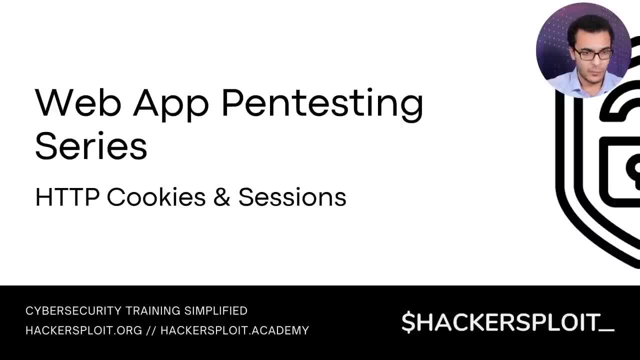 and sessions are, you know, elements of web applications and web app pen testing. that are, you know, quite important as you move along And you'll actually see how this ties into vulnerabilities like cross site scripting, for example. we're going to be taking a look at that. 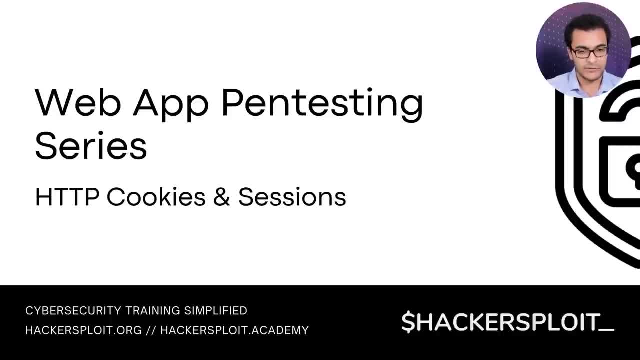 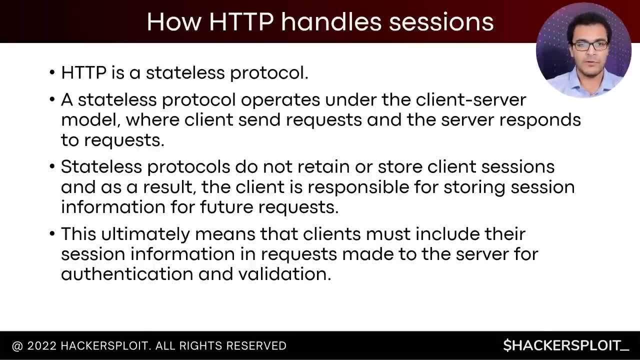 shortly, But before we get started with the practical side of things, let's get an understanding as to how HTTP handles sessions. All right now, if you remember, in the introduction video or where I covered HTTP, I mentioned that HTTP is a stateless protocol, right? So what is a? 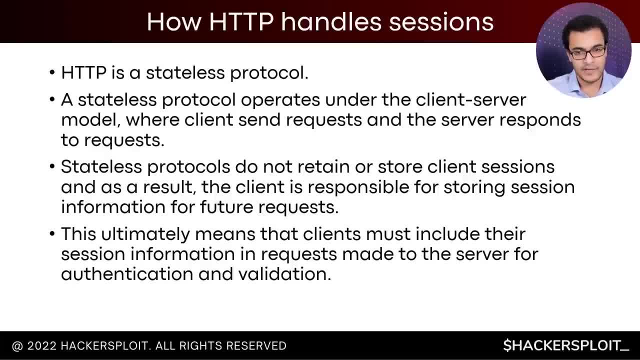 stateless protocol. Well, a stateless protocol operates under the same or the familiar client server model, where the client sends a request to the server And you know the server responds to these requests right. So you essentially ask for something and you use. you get whatever you asked. 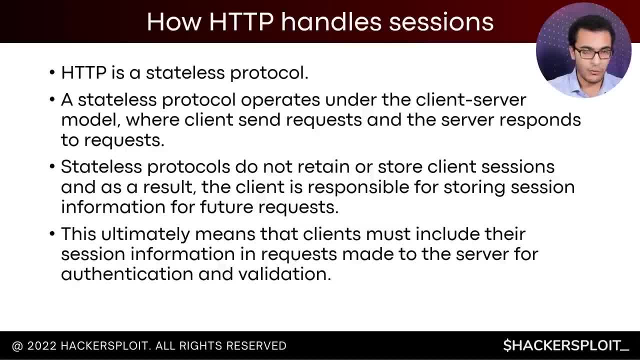 for Now, stateless protocols do not retain or store client sessions And, as a result, the client is responsible for storing session information for future requests. What does this mean? It means when you make a request you know to a website via HTTP. 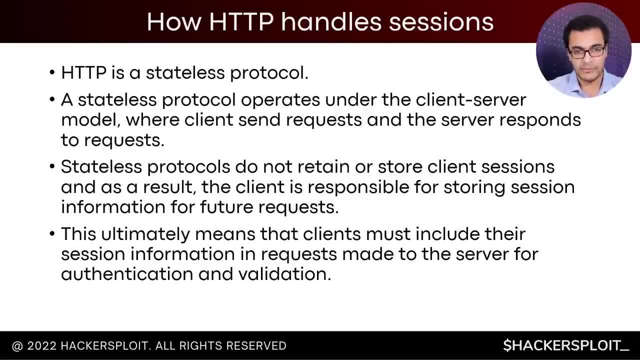 that is not stateless. So the problem here, as you can already tell, is what if the server you know needs some sort of validation or, is you know, wants to implement some form of session of session management, How does it do this, given the fact that HTTP is stateless? Well, this is where cookies come into. 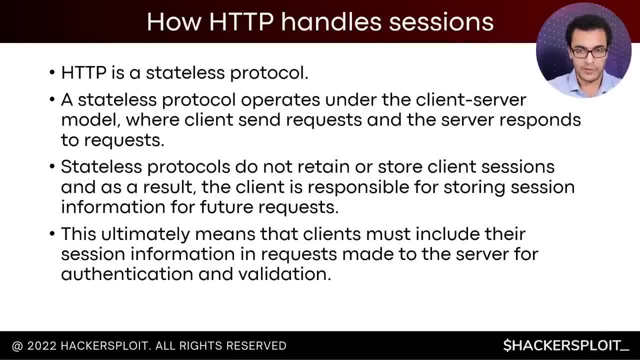 play right. So I'll get into cookies in a couple of seconds, But the the crux of this is that the client is responsible for storing information for future requests, Right? So this ultimately means that the client must include their session information in requests made to the server for. 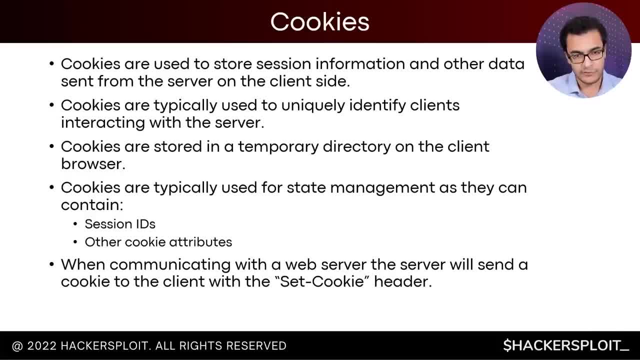 authentication and or validation. So this is where cookies come into play. So cookies are used to store session information and other data sent from the server to the client side. So I'll just use a simple example. Let's say I'm making a request to hackersploitorg, right? Well, when I make the get 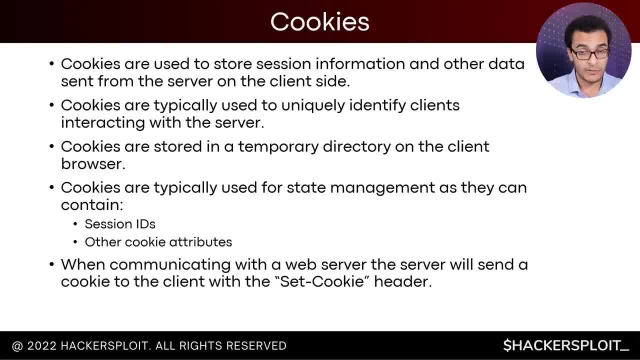 request. the server says: Okay, thank you for making the request. what you're looking for is available. But what I want you to do is I want you to set this particular cookie right. I want you to, you know, I want you to essentially set or save this cookie, this cookie, I want you to save it in. 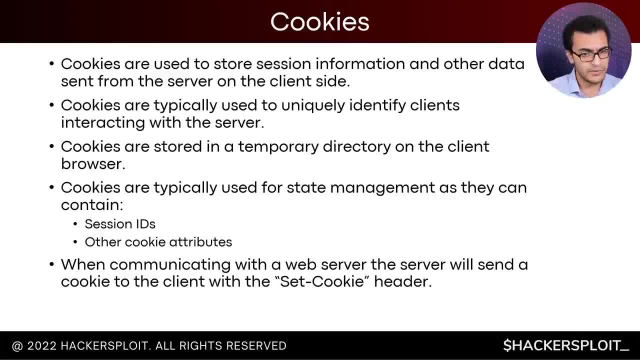 your browser. It'll essentially contain your session ID and a few other important things that are required from you when you reauthenticate Again. an example of this could be: you know your preferences for the website, So, let's say, you close a particular pop up. you know then that information is handled within your 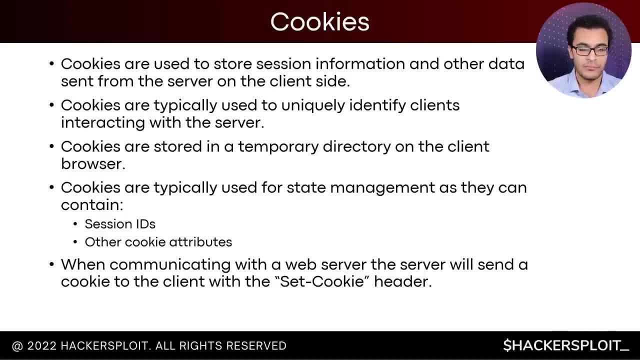 cookies that are stored within your browser so that the next time you make another request to that website or to that web application, your your preferences are stored in addition to your session information right Now. the way sessions are handled is something that we'll be exploring a little bit in this video and in a in a. 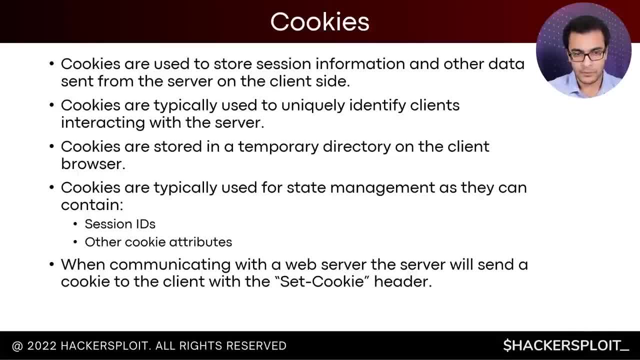 future video when we get to that point. So cookies are typically stored, as you know, in within your browser, right within a temporary directory. that's because on your browser, whether it's Firefox, Google Chrome, Safari, etc. you have the ability to clear your history, and under clear your history, you. 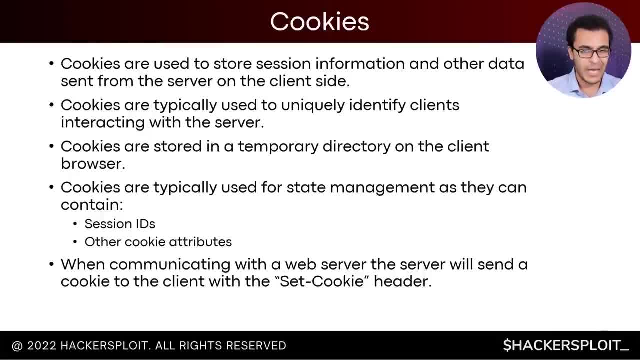 can clear cached content or you can clear cookies. Now, what happens when you clear your cookies from your browser? it means that, firstly, you'll need to log into all of the sites you're using previously. So if you've ever realized that- like, for example, if I'm signed into Google, then the cookie that that Google gives me essentially has a. 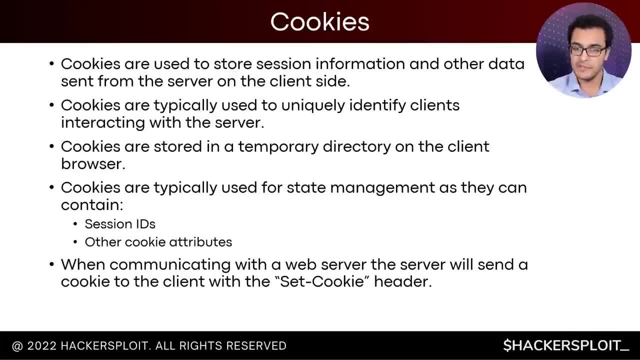 very interesting expiry attribute. That means that you know I can continuously open up my browser and I'm still signed into Google right Now when I delete my cookies. that means that you know all of that information regarding my. 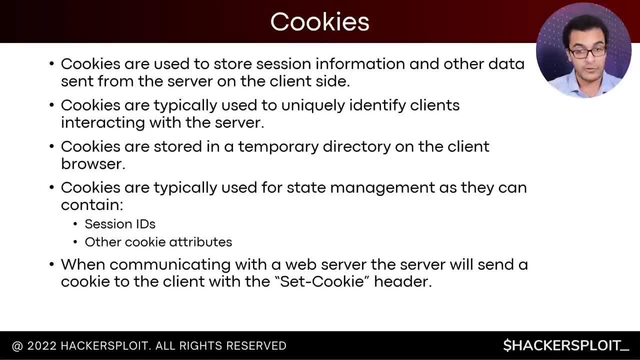 session is lost And, as a result, Google will say: okay, you need to log in again so that I can send you a new cookie. So cookies are typically used to uniquely identify clients that are interacting with the server And, as I said, they're stored within a temporary directory on the client. 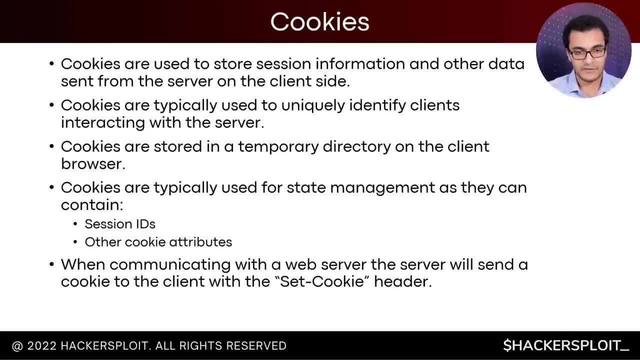 browser Cookies are typically used for state management, as they can contain session IDs and other cookie attributes that we'll get into shortly. So, when communicating with the web server, though, the web server will send a cookie to the client, or will send a response to the client with the set cookie header, essentially telling them what they need to what they need to. 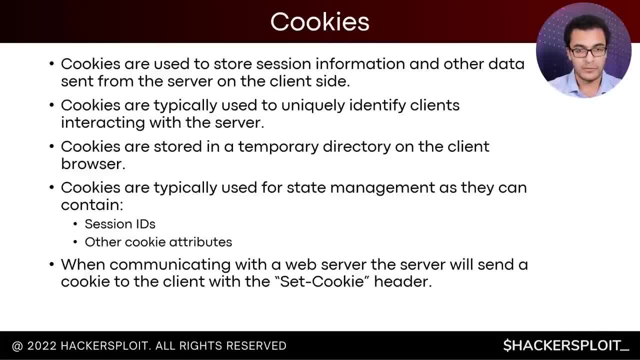 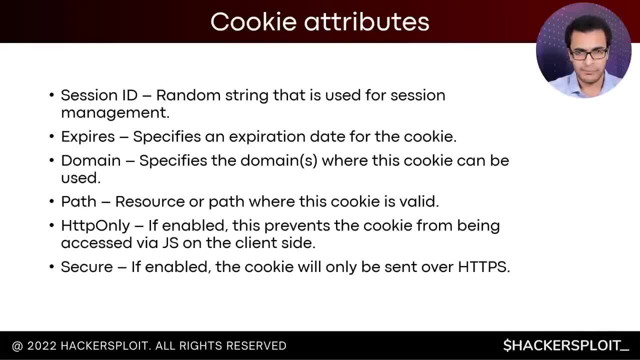 save, or, you know, providing them with a cookie that they need to save. you know the browser needs to save. So what are these cookie attributes? So what information is, you know, pretty much the most important when it comes down to a cookie. Well, 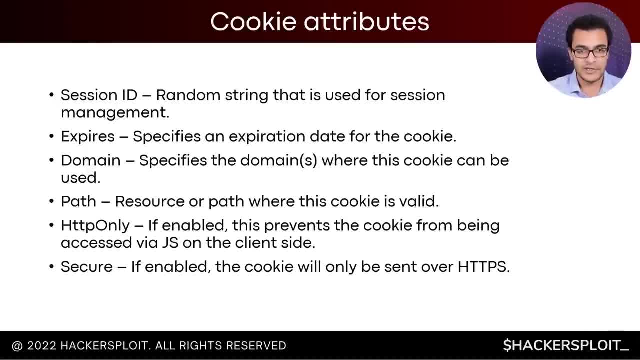 firstly, you may have a session ID. session IDs are essentially a random string that are typically used for session management. So an example of this is on the. if you actually try and access a web application built on PHP, you'll typically have something like a PHP session ID. right. 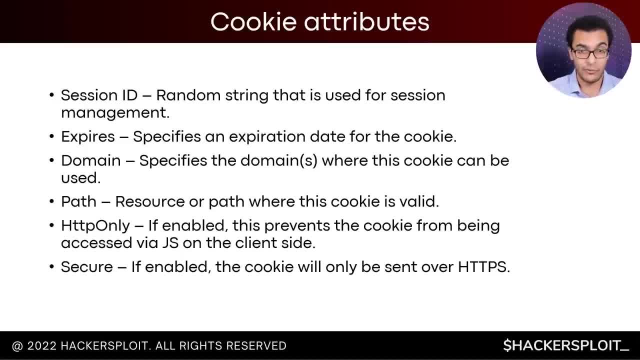 So that is used to uniquely identify you as a client or your browser for future interaction or requests that you may make. You then have the expiry attribute. Now this is used to specify an expiration date for the cookie. So this is: you know, the server will send this cookie, but the expiration date essentially states when this cookie should expire. 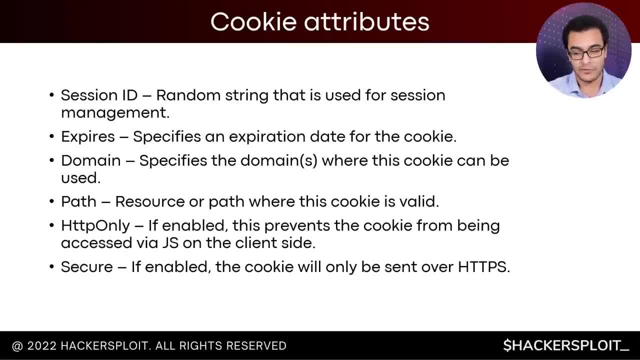 So, for example, if I have a website and I, you know, on the server side, I say that OK for all the clients, I want them, I want their cookies to expire after a week, right? So let's say, on the client side, now one of my customers logs into my website and you know, they get the cookie. 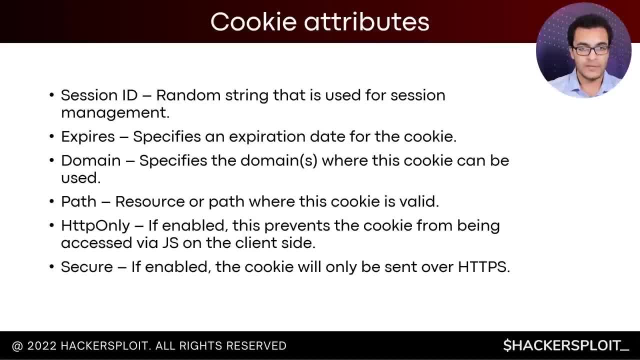 It's stored within their browser And, you know, throughout that week they can continuously open up their browser and you know they can access the site without having to log in. However, after the expiration date, or when the expiration has lapsed or you know, the validity period for that cookie has lapsed. 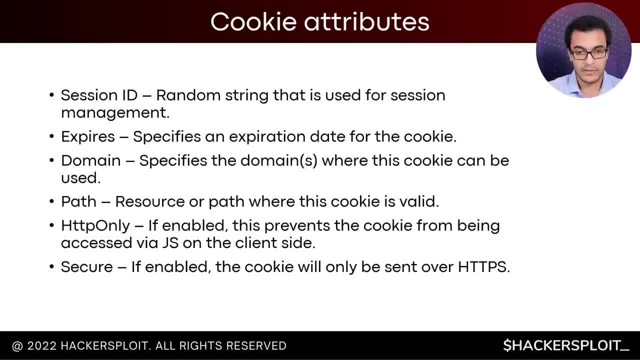 then I'll need to log in again to get you know another cookie. You then have the domain attribute. This specifies the domain or domains where this cookie can be used or where it's valid. You then have the path. This is used to specify the resource or path where this cookie is valid. 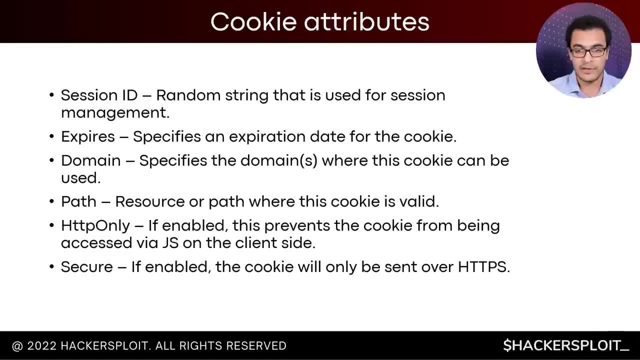 So you know the URL, you know it could be to a particular directory, maybe a specific dashboard or for a specific file. You then have the HTTP only attribute. This is really, really important. This is one of the areas I'll be focusing on in this video. 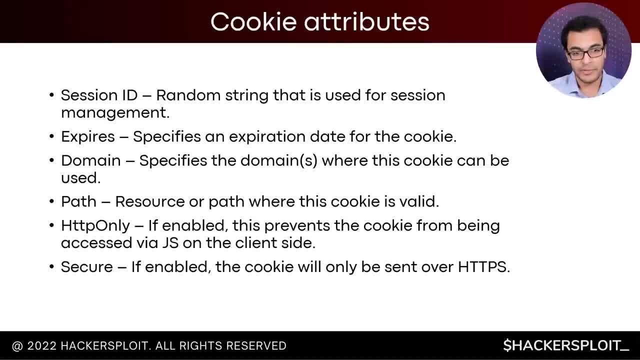 So if this attribute is enabled, this will prevent the cookie from being accessed via JavaScript on the client side. You'll actually see this and you know why this is so important and why this is typically enabled on a production site. You then have the secure attribute where, if enabled, the cookie will only be sent over HTTPS. 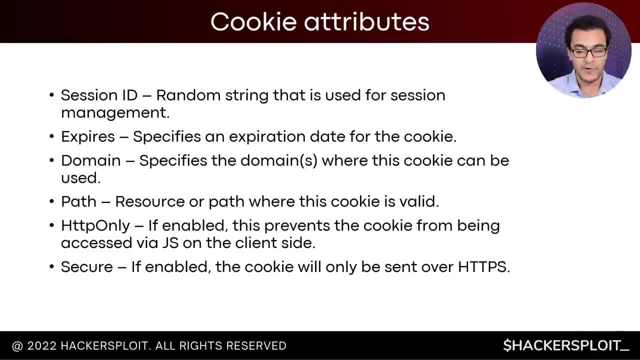 Again, that's quite useful, Very, very important, because if a cookie contains- you know, if it contains- a session ID, then if it's sent over HTTP which is not encrypted, then a man in the middle attack can essentially sniff out those requests and identify your- you know your session ID or pretty much your entire request with the cookie. 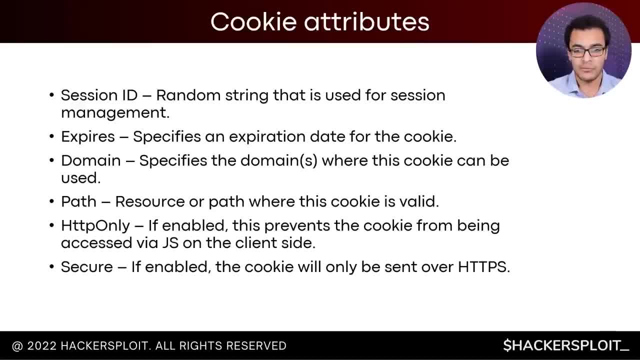 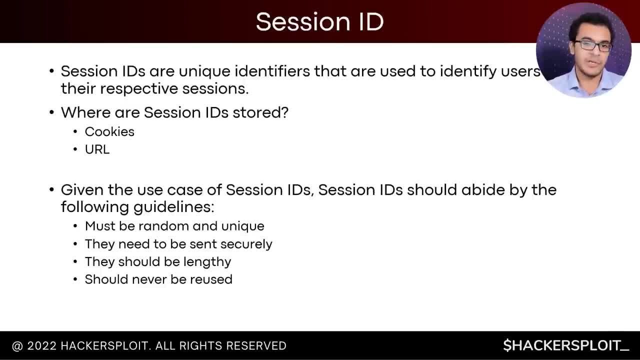 you know information itself. Consequently, you know, you get the idea. Attackers can then, pretty much you know, perform impersonation et cetera. So I mentioned session IDs quite a lot. So what is a session ID? 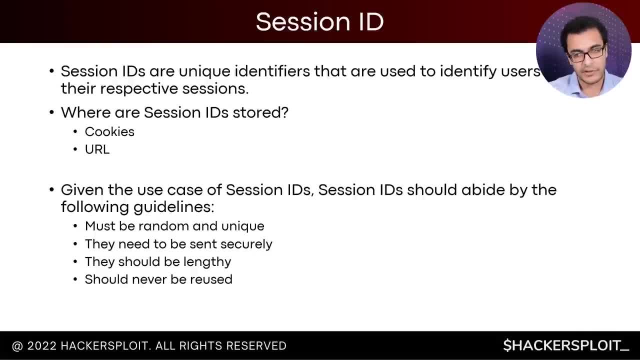 Well, session IDs are unique identifiers that are used to identify users and their respective sessions. So where are session IDs stored? Session IDs are typically stored in two primary areas. I've not mentioned the other ones, but these are the ones you'll typically see. 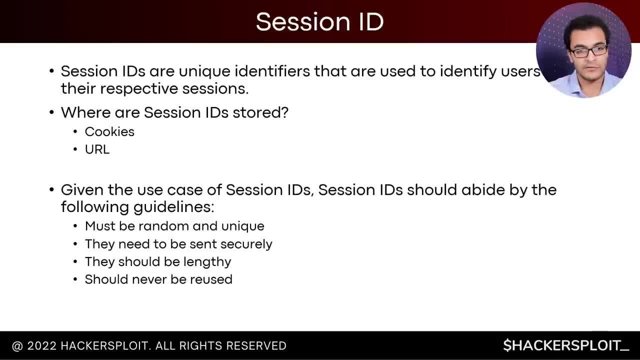 see. So the most common one is they'll be stored in cookies or, you know, as a URL parameter. So if you've ever seen within your browser or- let's start off with cookies- So if you've ever intercepted a request with Burp Suite, you might have noticed that this, the session ID, is stored. 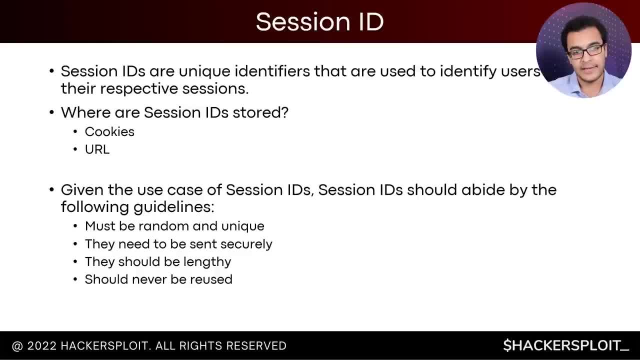 within the actual cookie right or the cookie content. And then, in the case of URL, again the same, the same concept applies. if you've ever logged into a site- most likely a PHP site- in the URL you might have noticed that you have a PHP session ID, you know parameter. 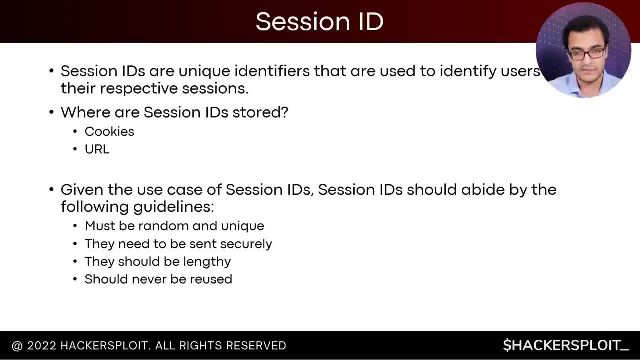 and the value has the PHP session or the actual ID itself. So there's multiple ways that they can be stored. Now, one thing that I wanted to point out is, you know, given the use case of session IDs, session IDs should abide by the following guidelines. So 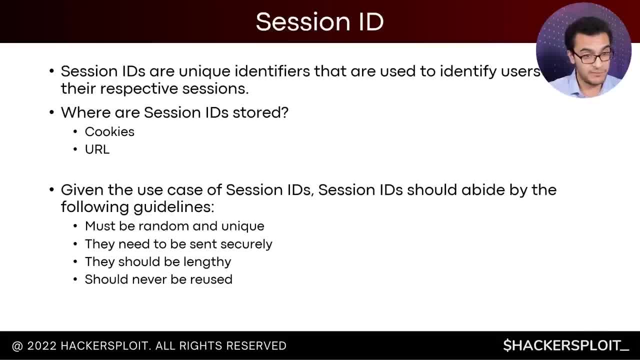 you know, from the perspective of security, session IDs should be random and unique. they need to be sent securely, So over, you know, a secure and preferably an encrypted tunnel. So you know, HTTPS, TLS, etc. And they should be lengthy and should never be reused. 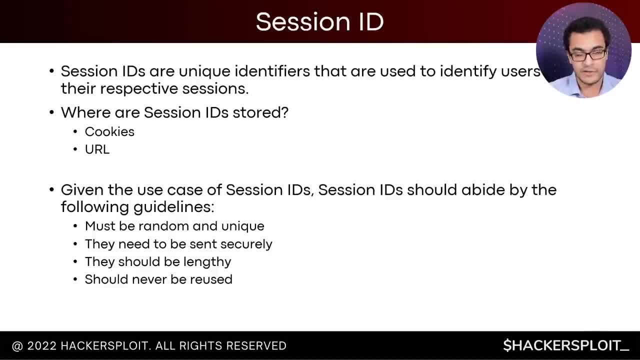 So you know, given the fact that we know session IDs are used to uniquely identify users, then of course they need to be random and unique, So other users should not be able to guess them or should not be able to essentially identify or, you know, get that. 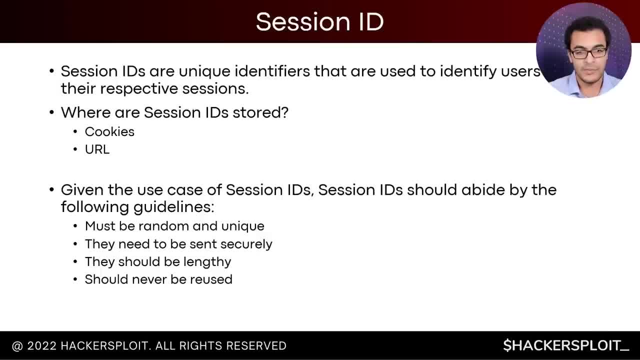 session ID under any circumstance. they need to be. they need to be secure from man in the middle attack, So that means they need to be sent securely. they should be lengthy. that ties into the the old concept of them being random and unique and should never be reused. So two users. 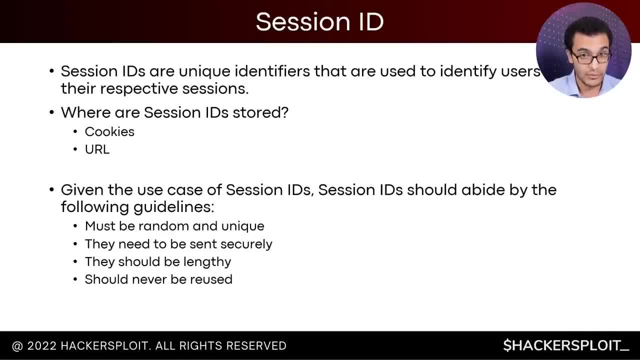 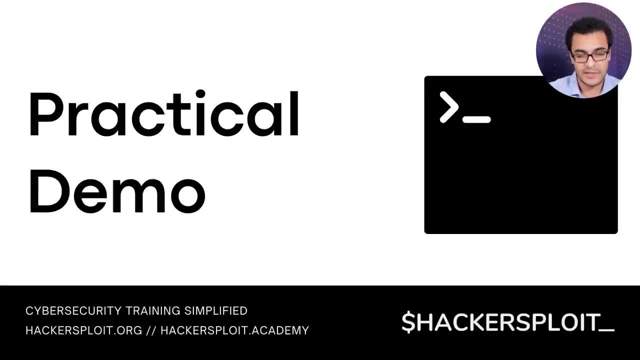 should never have the same session ID. you can pretty much guess the problems that that would cause. Okay, so now that we have an introduction to cooking cookies and sessions or session IDs, let's take a look at, you know, a practical example. So we're. 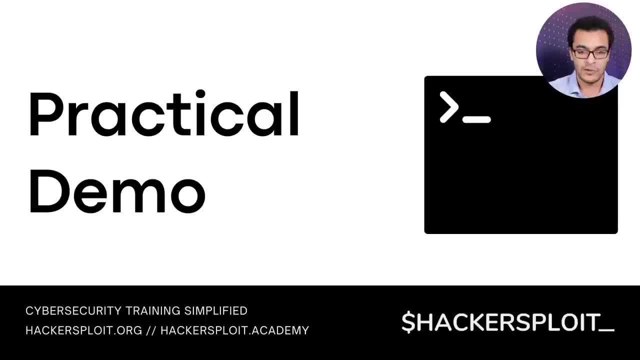 going to be utilizing the damn vulnerable web application, So I'm running it within the Docker container. If you check my previous videos, you'll actually- you can actually learn how to set it up yourself with Docker. it's really cool And I'll walk you through a few, a few interesting aspects. 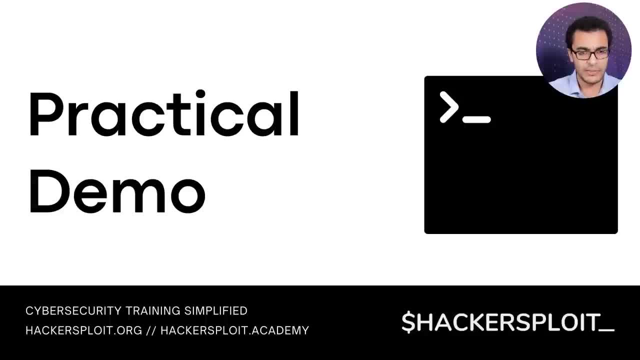 of cookies and session IDs and show you what I mean from a security perspective And from the perspective of an attacker. you will be able to get a better understanding of how cookies can be exploited and where they apply. Alright, so let me just switch over to my Kali Linux virtual. 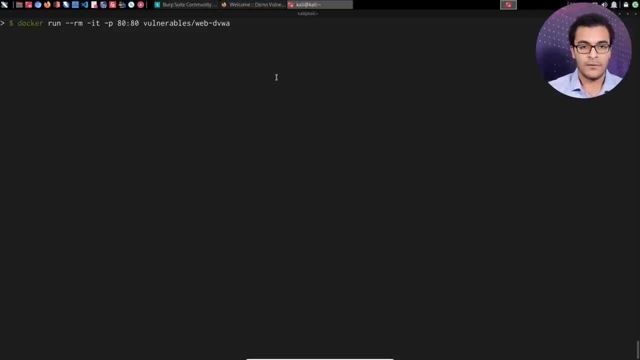 machine. Alright, so I'm back on my Kali Linux system And I'm just going to start up the Docker container. So this is the vulnerable, damn vulnerable web application And I'm just exposing it on port 80 locally. So I'll start it up And we'll give this a couple of seconds And of all. 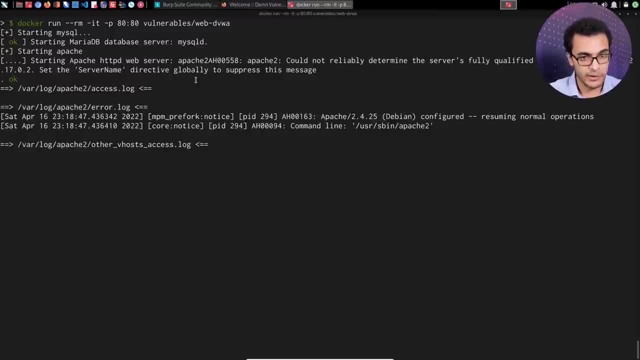 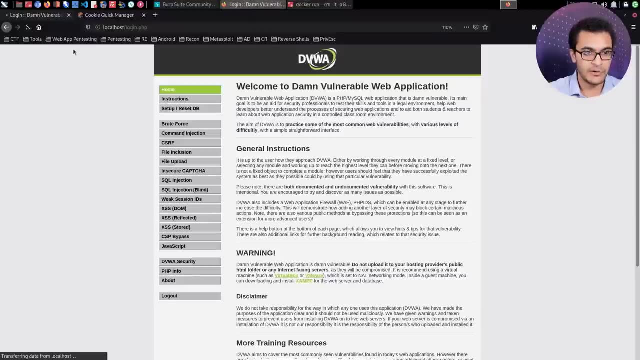 the things that we've done. we've already started burp suite, but intercept is disabled for now because I want to explain a few things. Right, so that should be working. So let me open up my browser. I should be logged out And we'll just close that. Alright, so it's working. Now we need: 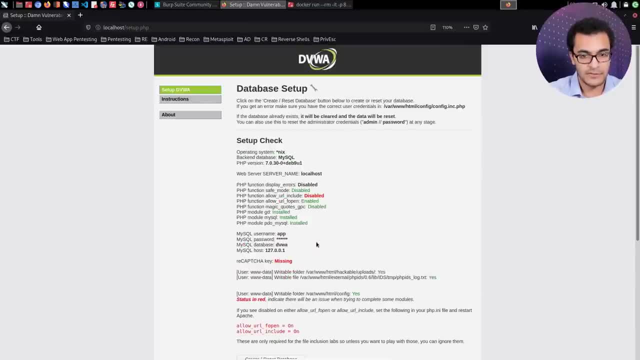 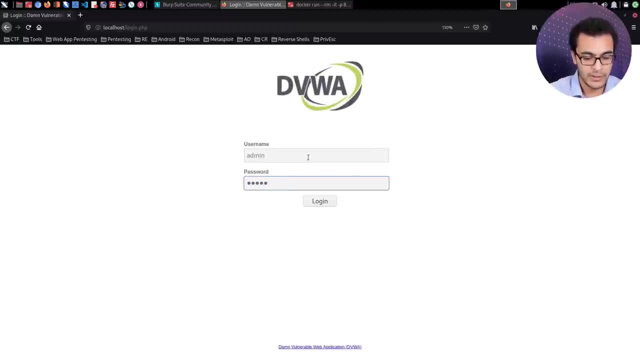 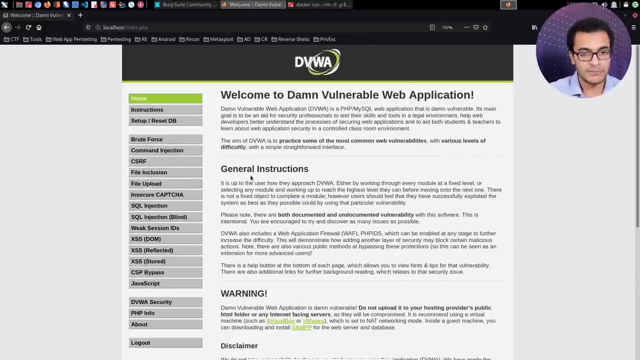 to create the database. So setup dot PHP And I'll just say create the database here And I can then log in. So the default credentials for the damn vulnerable web application are admin and password. Alright, so let me log in There. we are Fantastic. So you know. very simple web application we should have already. 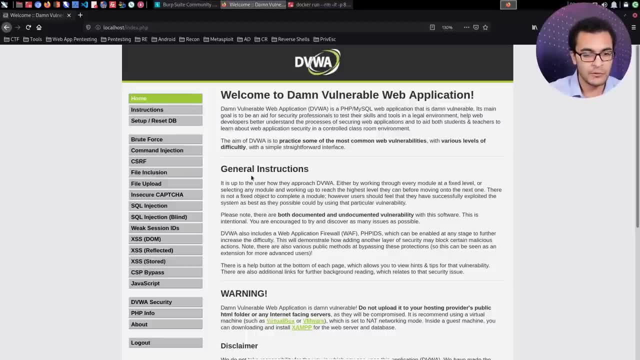 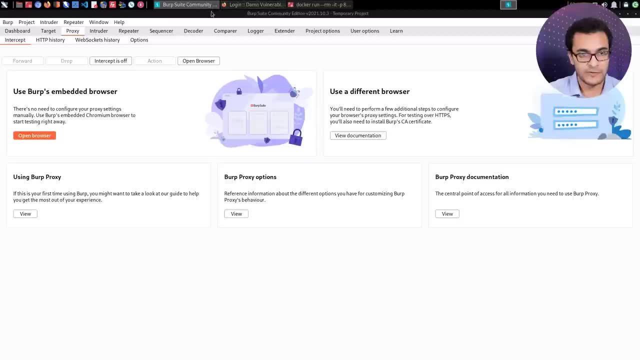 have a cookie, But let's take a look at it from the beginning. So what I'll do now is a logout. you might be a little bit confused, but don't worry. I'll just enable the burp suite profile with Foxy proxy here And I'll intercept. enable intercept on burp. And let me just refresh the. 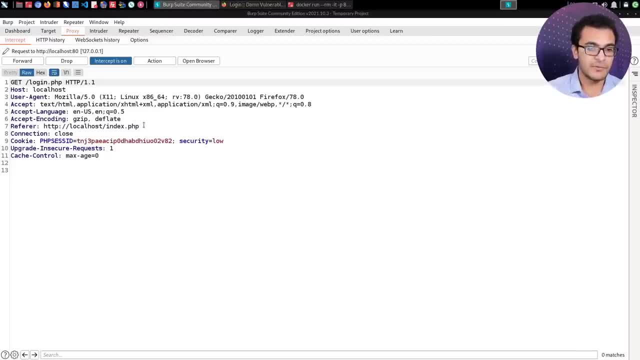 page. So you can see, when we make the get request, the server will respond with the cookie that we should use Now. the cookie in this case contains the PHP session ID. So what's happening here is we've requested for the page itself, or, you know, we've. 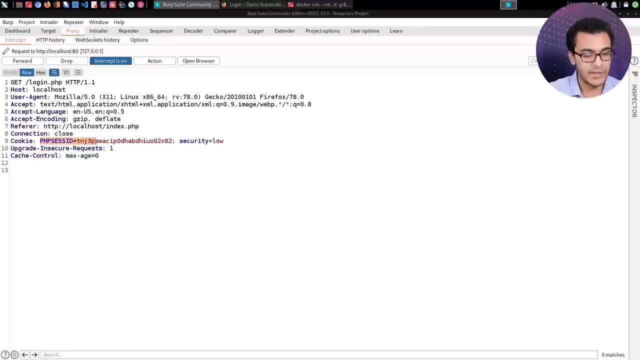 essentially trying to access the site And the server has responded and it says: Okay, you can access the site, But I want you to save the following cookie: So PHP session ID, and then it gives you the unique, you know- session ID, And then we have another one which is security. So 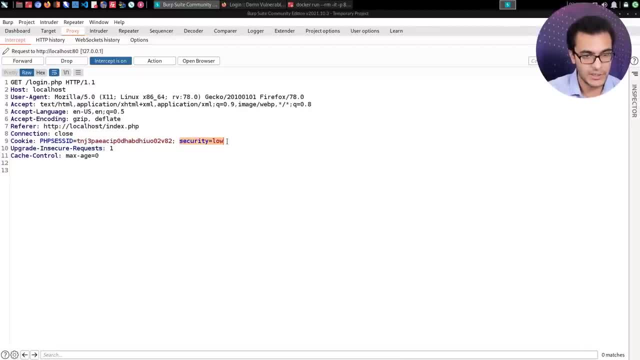 this is another additional piece of information that is being passed, or, you know, being passed along by the web server in this case, because this is the damn vulnerable web application. this is used to specify the security level. So from this point, you know, we can pretty much 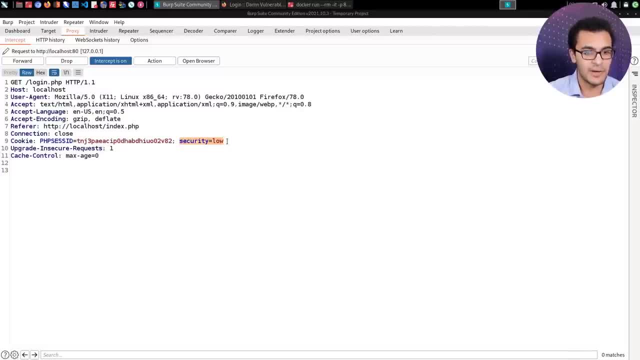 customize or modify it, But you know that's really not going to affect the application itself. we're just going to be able to increase the security level etc. So again, just to make sure that you understand, this is not. this is not reflective or related to how applications will. 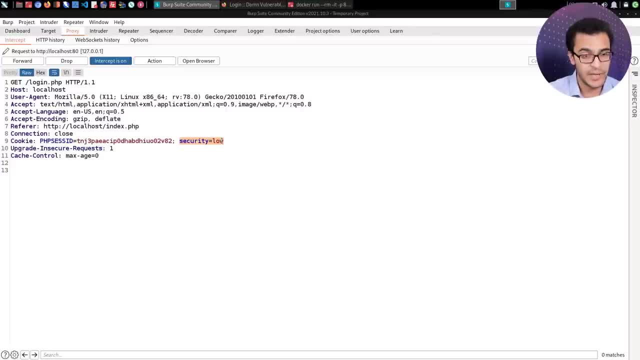 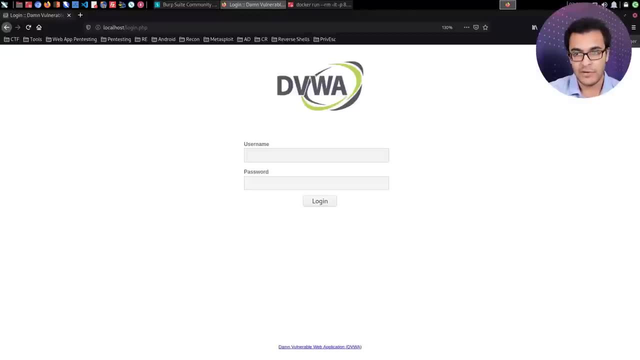 typically, you know, utilize cookies. This is just in the case of the damn vulnerable web application. So I'll just say: Ford, okay. And if we click on cookie manager? cookie manager is a really cool Firefox extension or plugin, whatever you want to call it. it allows you to manage, edit. 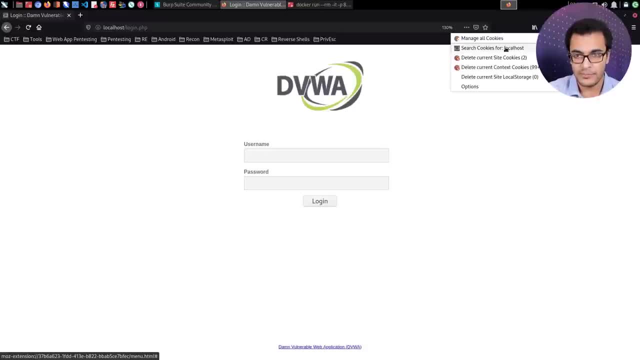 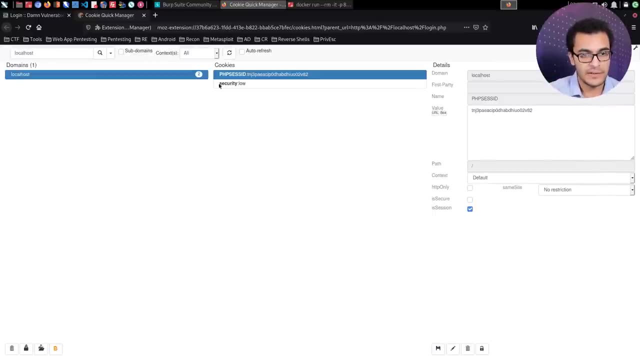 manage and edit your cookies for different sites. So I'll just open up, I'll say search cookies for local host, because I'm hosting this locally, And you can see that this is the cookie that is stored for the following website. So the cookie has, you know, the following attributes, and then it has: 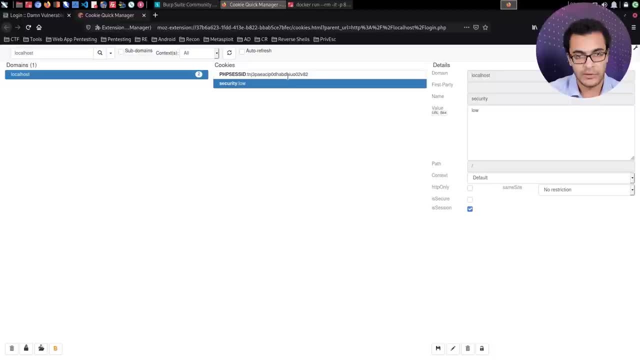 the additional information. In this case this is the second one, So security low, But for PHP you can see. these are the two cookies here. So PHP session ID, that's the cookie. You can see all the attributes here, which I'll get to in a second. However, if we now try and 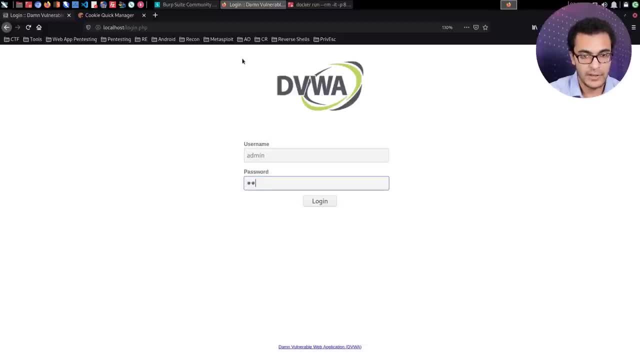 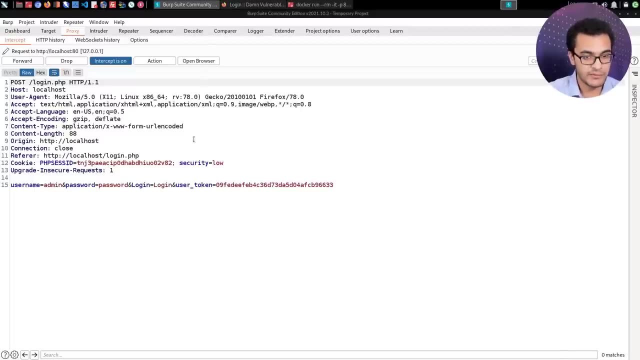 log in now with the, with credentials. I'll just say admin password. right, I'll just say login. You can see that the browser, the web server, now says: okay, you want to log in. for your login, I want you to use the following session ID: Now you might be a little bit. 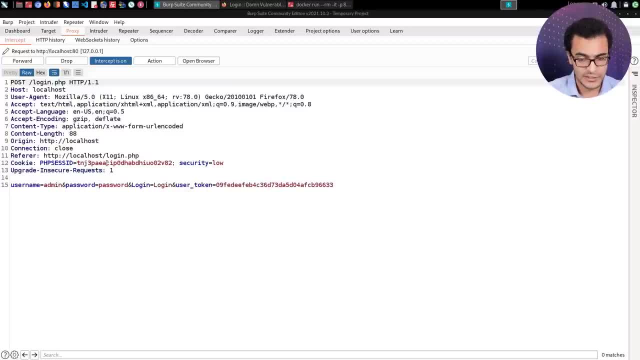 confused If you, if you, if I told you that session IDs are used to track, you know are used for session management, you might be saying: well, I, we didn't log in yet. Why did we get a session ID previously, when we were anonymously browsing the site? Well, that's because session IDs can be for. 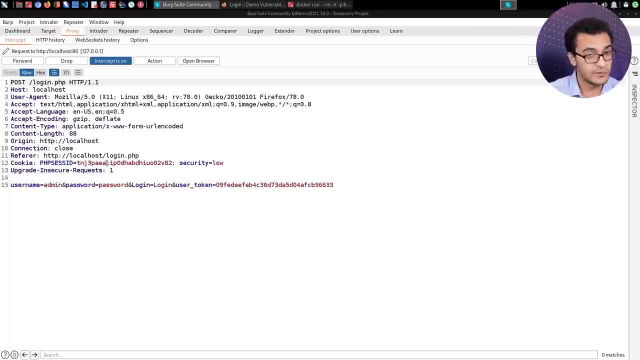 both can be used in both ways. it can be used for anonymous users, where it's really non consequential but still very useful in tracking your session, And then, of course, you can also it can. they can also be used well for authenticated session management. So just take note of this cookie here, right? So TNJ3PA, So. 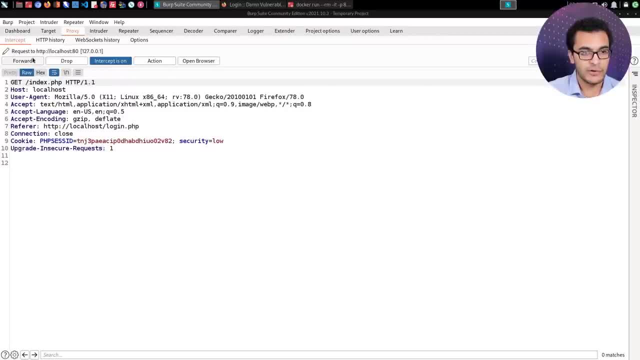 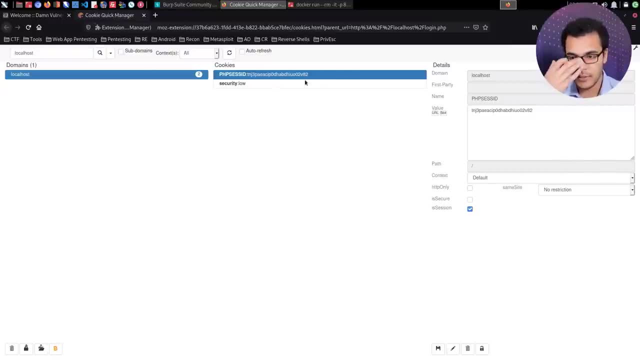 I'll just say forward And you can see the same one there. So forward, forward, and we click on the cookie manager. here you can see that the it's the same cookie. sorry, it's the same session ID here. Alright, so we're now logged in. 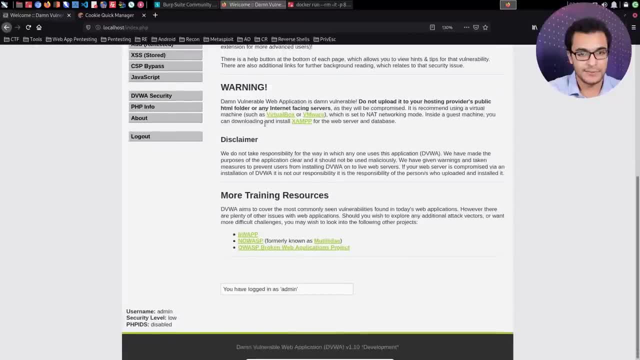 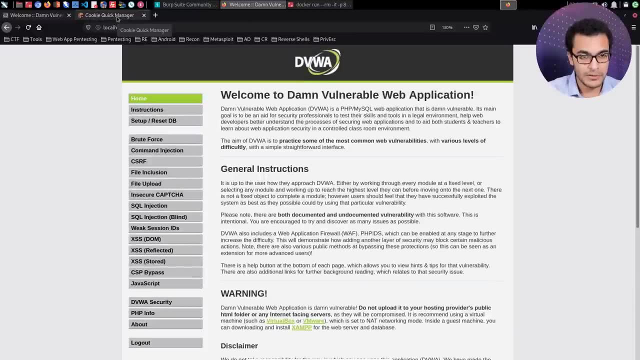 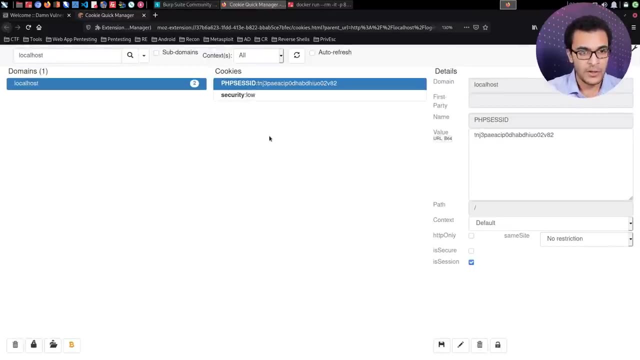 Okay, we're logged into the damn vulnerable web application. Nothing special there. What I wanted to highlight was a few things. So I'm not going to be utilizing the cookie manager, because you can really do a lot of cool stuff here. So the 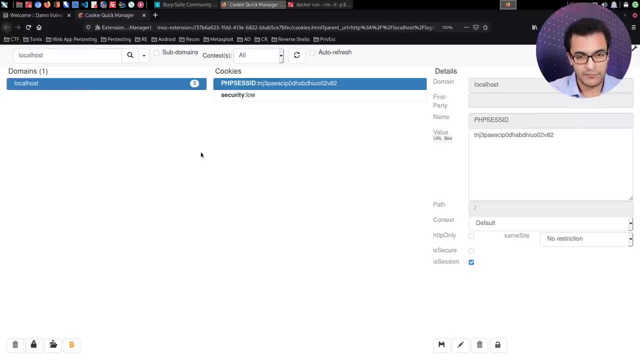 cookie manager. you should be able to see all your other sites that have cookies here, But in my case, I cleared all of them because I wanted to explain this. So this is our cookie here. Alright, so you can see. these are all the attributes we. 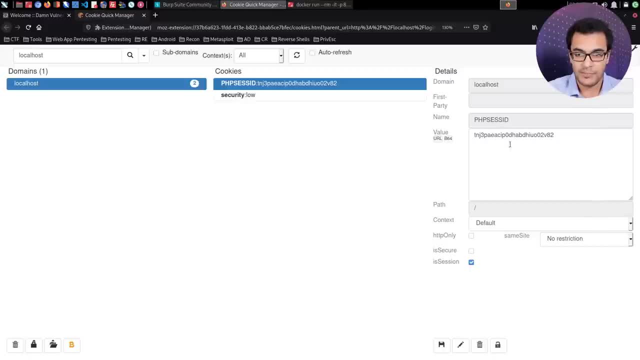 have the domain, localhost, the name of the cookies, PHP session ID. that value is specified in here. you have the ability to decode it with: to perform URL decoding, which I'll get to in another video, and then base 64 decoding. In this case the session ID is random and 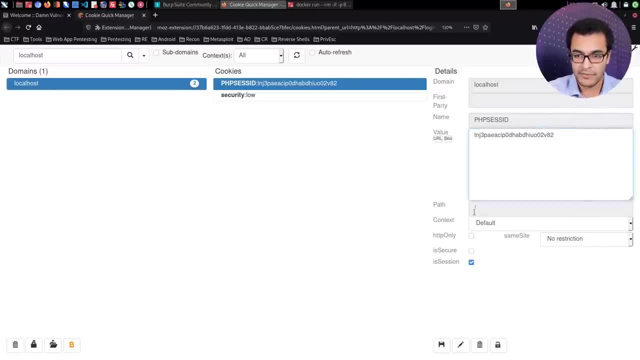 it's not encoded And, so far as I know, you then have the path, the context, etc. Right, But what we're interested in here are these three, or rather, yeah, these three. So you can see at the bottom that this attribute is session, And I didn't cover it in the slides for a very important reason: is enabled or it's. 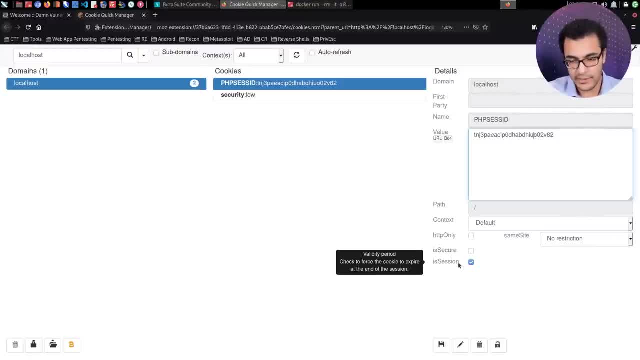 checked. So what does that mean? As you can see, if you, if you highlight or you hover over this, it'll tell you that, if enabled, this will check or will force the cookie to expire at the end of the session. Now, the great thing with cookie manager is we can modify all of these. 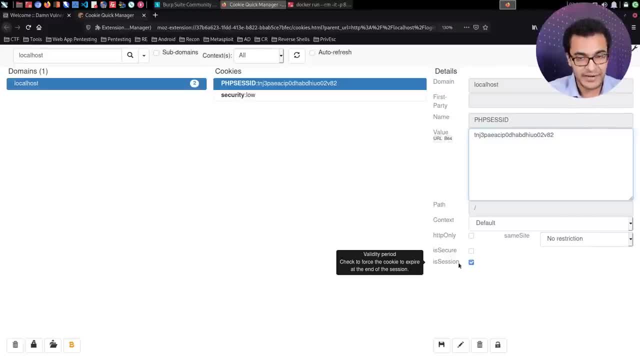 attributes and consequently change the way we interact with the web application. What do I mean? Well, if I disable is session, I can specify another expiry date. But before I do that, I want to show you that this does indeed work. So to 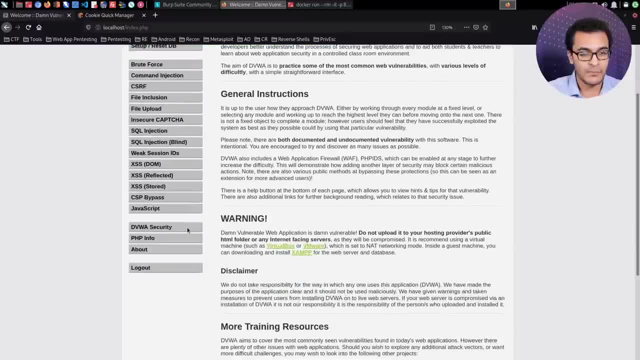 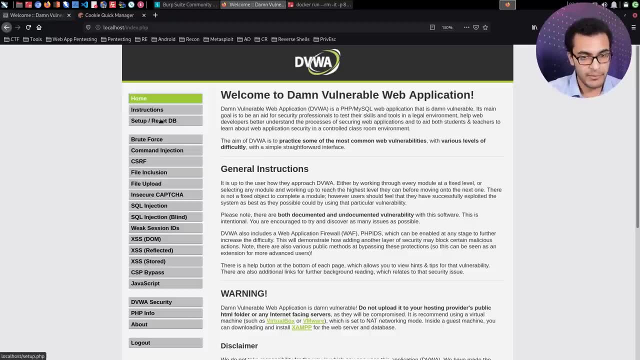 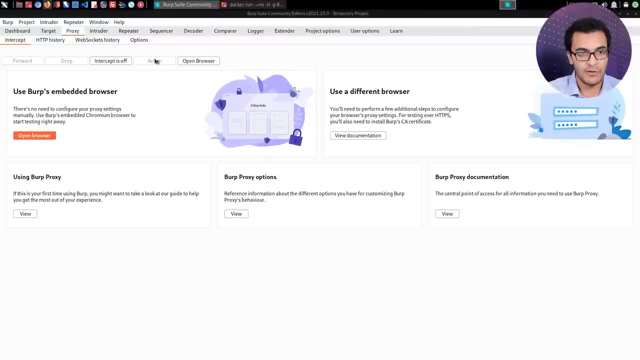 show you that this works. I'm just going to, I'm just going to close my browser, right? So because it's it's currently checked, that means when I exit from my browser I'll need to log in again to the damn vulnerable web application. So I'll just say close tabs and I'll open up Firefox. 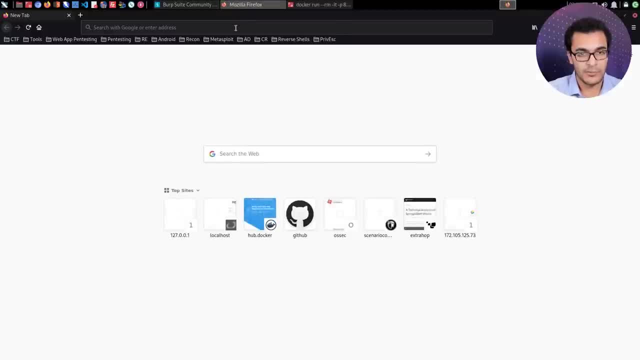 again, right, And we'll give that a couple of days, A couple of seconds. So I'll say localhost. You can see I need to log in again, So I'll just log in one more time. There we go, And now let's modify this. 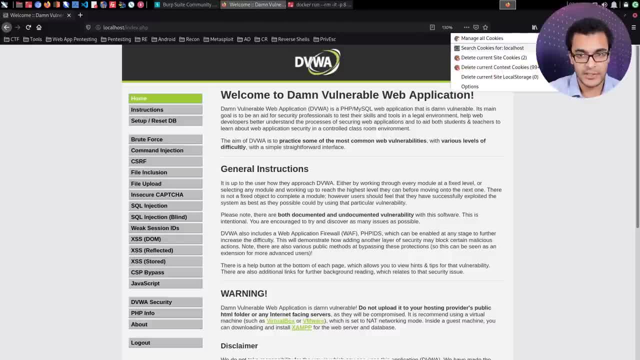 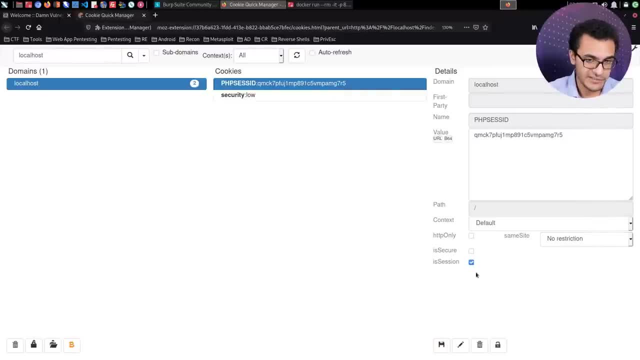 cookie. we should have a different PHP session ID right. So search cookies, you can see it's now different because our session is different. So if we wanted to persist the same cookie, then we can disable is session and set a different expiry date. So I can say: I want. 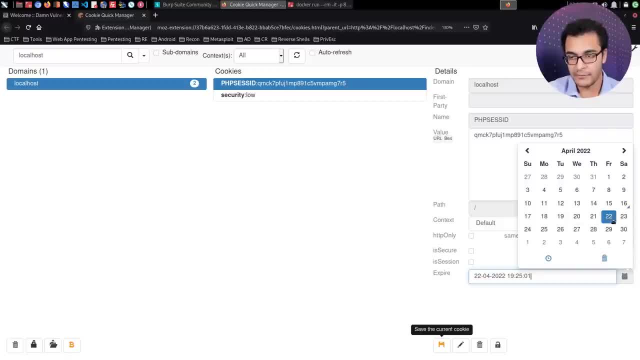 this to expire on maybe Friday Of you know, the 22nd of April on Friday. I can then save that. I need probably need to save that again. So 22nd, there we are. save it, Alright. so now that we've saved it, we have essentially modified the cookie attribute to say or to essentially state to the server that hey, I have the following cookie. it doesn't expire till the following date, So please give me access, Alright. so let's test this out. 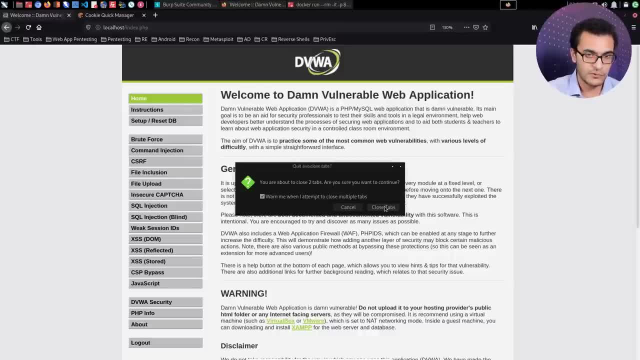 And we'll see if it works. so remember, i'll just close up my browser. this will. this is what you'll typically see, as i said, with a site like google or facebook that maintains your session, or you know, the the validity uh of the actual cookie itself uh have a specific date. after a while you may be forced to log in. 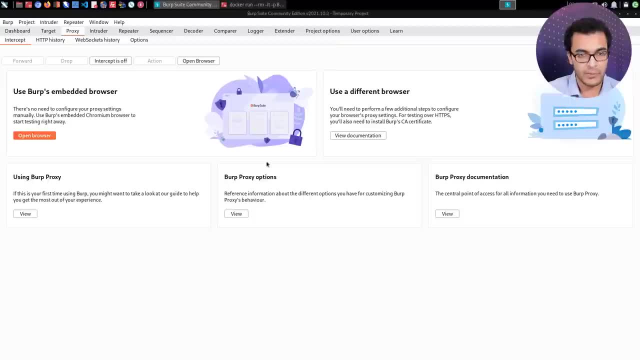 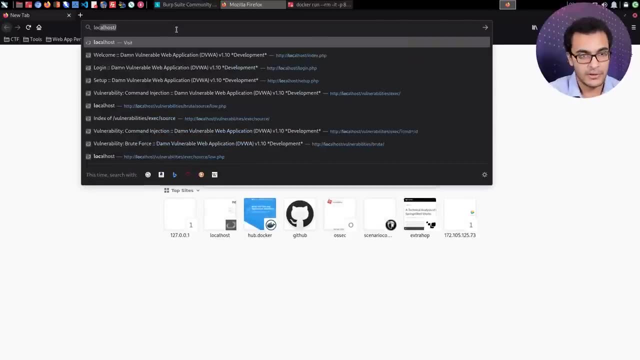 again, but that's based on the actual company that set up that website, so i'll start it up again and we'll just open up a localhost again. remember i shut down my browser completely. there we are, so we're now logged in. we don't need to log in again, so 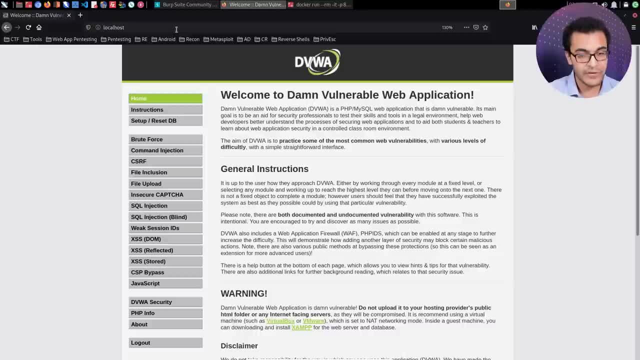 i again. the reason i'm showing you this is to show you that cookies are really, really they. they play a crucial role when it comes down to session management and the way the client interacts with the server, and vice versa. okay, so let's take a look at the cookies again. so i'll 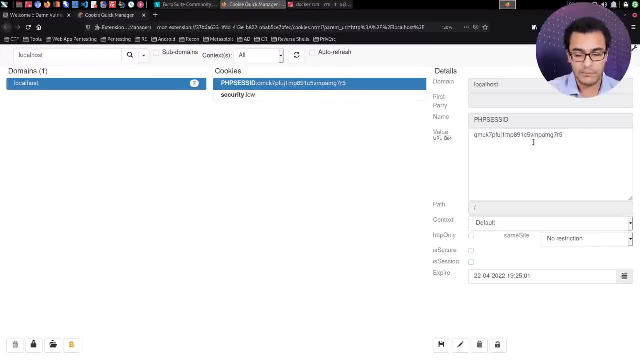 just search cookies for localhost, you can see it's the same one. now let's take a look at some of the other attributes. some of the other attributes: the one that i wanted to cover is the html, and the one that i wanted to cover is the http. um, the http only attribute. so this is a theft. 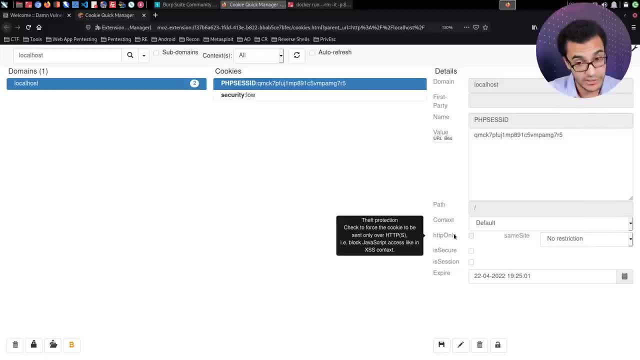 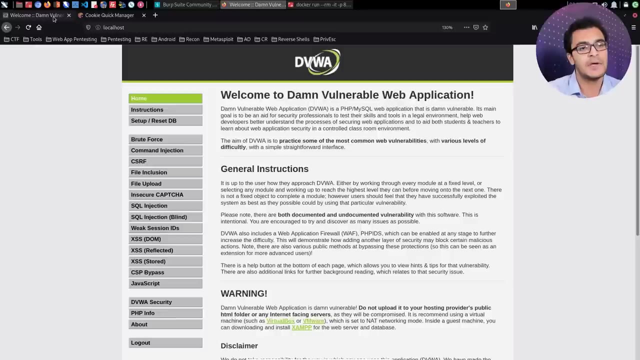 protection. so this will check to force the cookie to be sent only over http or https. make sure to note that. so what this does? it is it essentially blocks javascript access, like in cross-site scripting context. what on earth does this mean? well, you can see it's currently unchecked which. 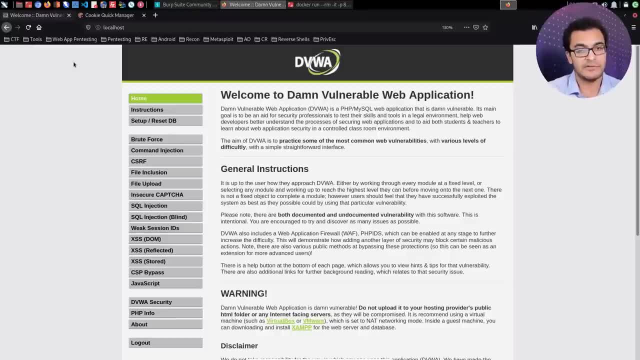 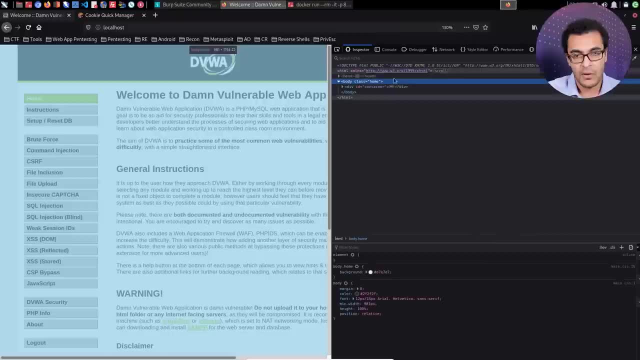 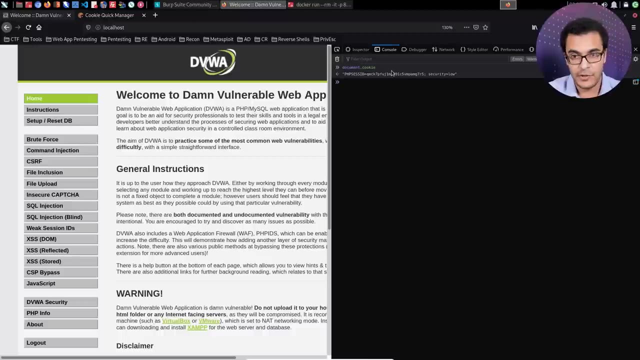 means that on the client side i can pretty much utilize javascript to to interact with the cookie or to get the actual cookie. so if i inspect element here and i head over into the console, i can use javascript to say document dot cookie and it should display it. so there we are. it actually displays the cookie there. so php session id security equals low. 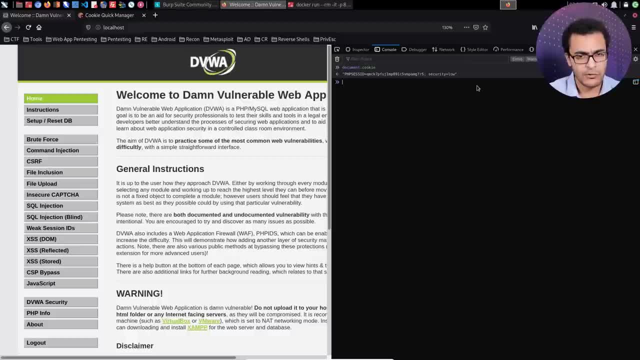 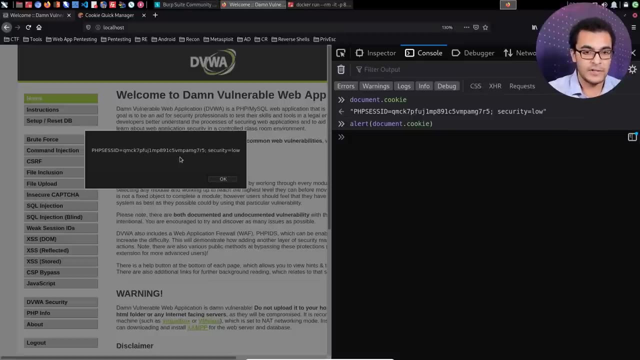 all right, and an attacker. you know, and i'll walk you through this with cross-site scripting. but you know we can essentially say alert, uh, alert, and within this we can say document, uh. i don't know if you can actually see this, let me just zoom in. so document, dot cookie. if i hit enter, you can see. 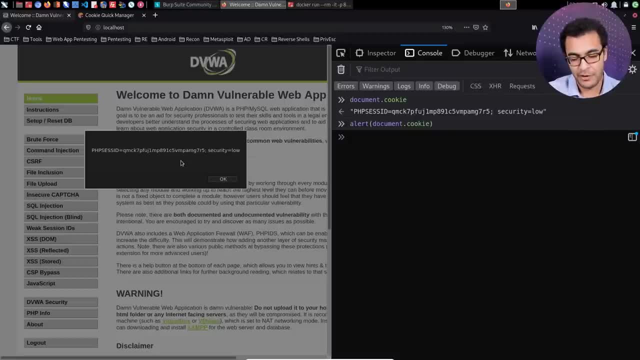 that this is typically what you know. uh, you, we, we would now be getting into the territory of cross-site scripting, and i'll actually show you a practical example where this could potentially be dangerous and why that needs. all that always needs to be checked on a secure site, so you get the idea. 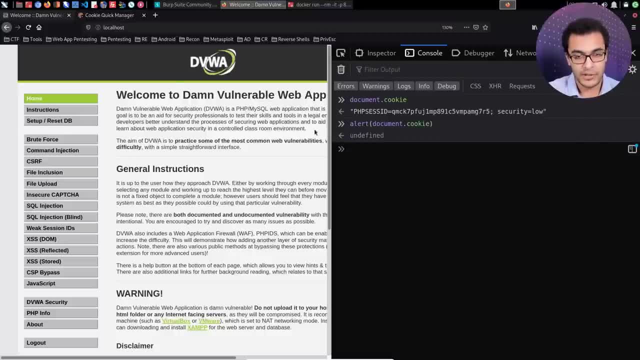 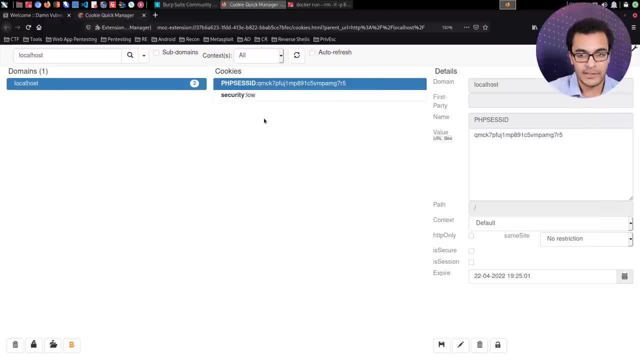 when that attribute is not checked or enabled, then we can pretty much, through the client side, interact with the cookie via javascript. so let me go back in here and, uh, what i'll do now is: let me just check that, so i'm gonna save it. there we are, so that's saved, uh, and now let me just uh, we can refresh the page that. 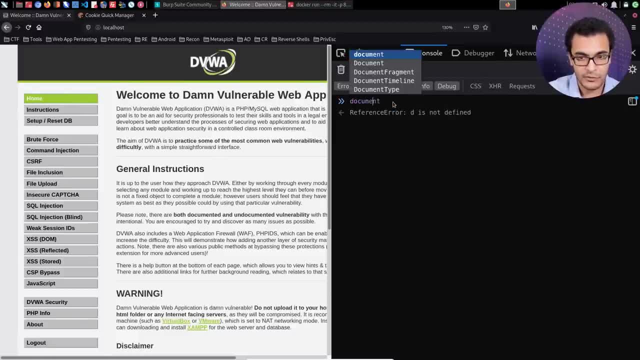 shouldn't affect too much of the functionality. but if i now say documentcookie, you can see we now get a, an empty string, or you know we essentially get an empty value there. so you can actually see how this is helpful. and if we repeat our previous example where we try and generate an alert box, you can see doesn't display it. so you might be. 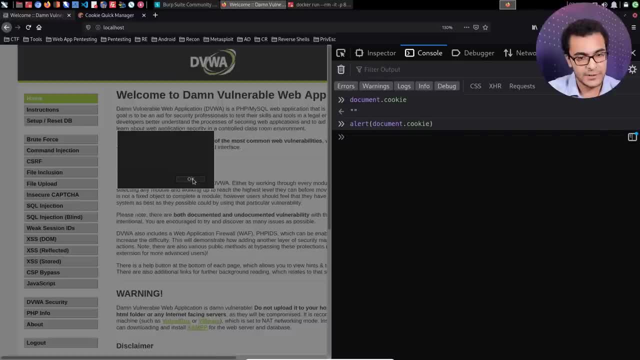 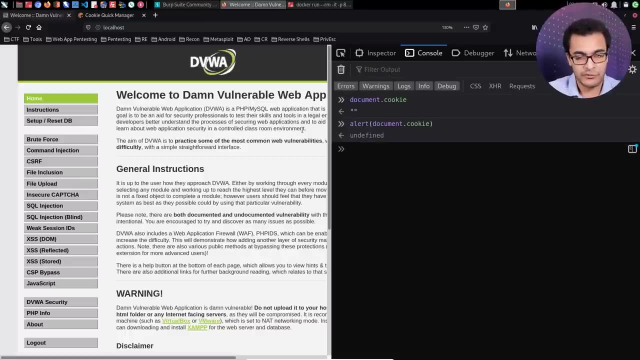 asking yourself: well, that's really interesting, alexis, but how does this tie into web app pen testing? well, i'll show you in a couple of seconds because, as said, these set of introductory videos are explaining a lot of the foundational stuff that a lot of people ignore. but if you understand, 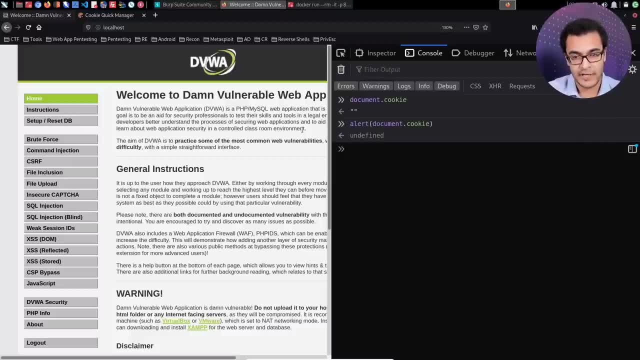 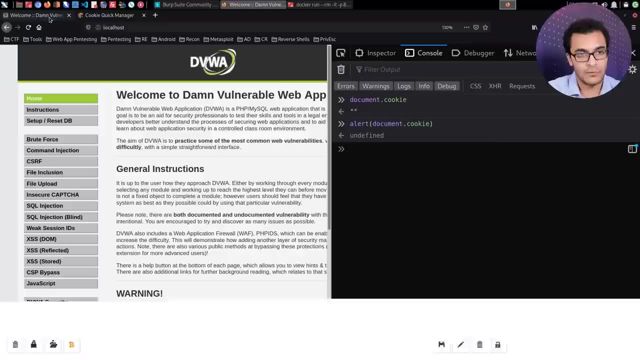 it, things like cross-site scripting become much easier to understand, things like cross-site request, forgery, etc. so what i'll do now is: let's- uh, let's go ahead and uncheck it or disable it, right, and uh, there we are fantastic. so i'll just go back in here and let's go into cross-site scripting stored. 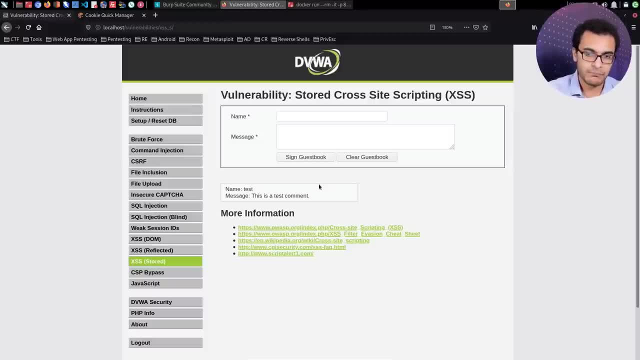 all right. so you understand pretty much how this works. this vulnerability essentially allows a potential user to essentially in this, in this context- inject javascript code into the actual web page so that when other users, um, when other users access that page, that javascript is executed on the client side. now you might be saying, well, how is that useful? 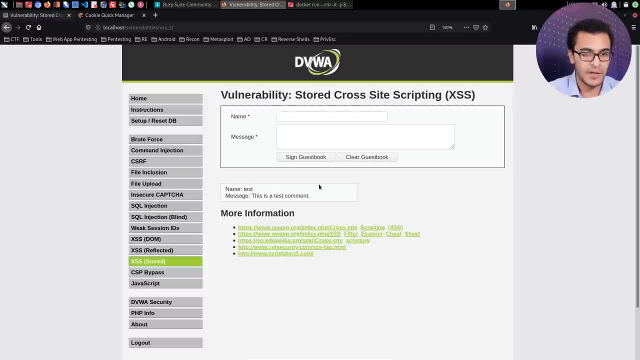 from the perspective of an attacker. well, if you customize the javascript, you can actually have it. uh, send the the information of the other user who is accessing that page to you, for example, you can steal the, the actual cookie itself, the php session, all of that good stuff. so let me show you. 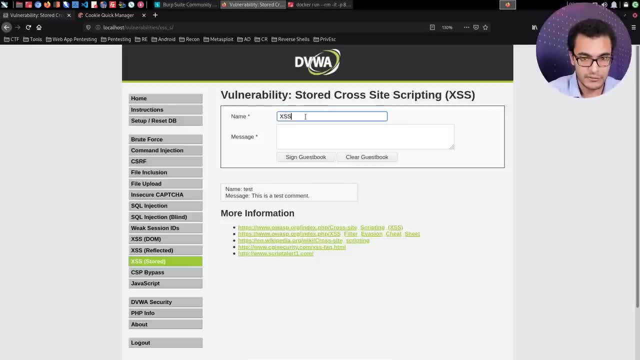 through a very simple example. so i can call this one: uh, we can just say cross-site scripting, and within here i can say script um, and i can say alert- let me put this in brackets here. so document dot cookie, all right, and we just close that uh, script tag there. 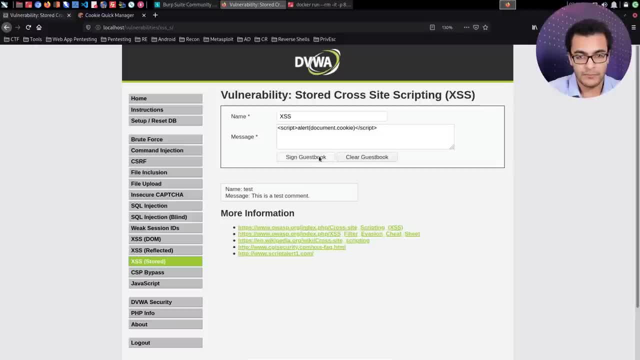 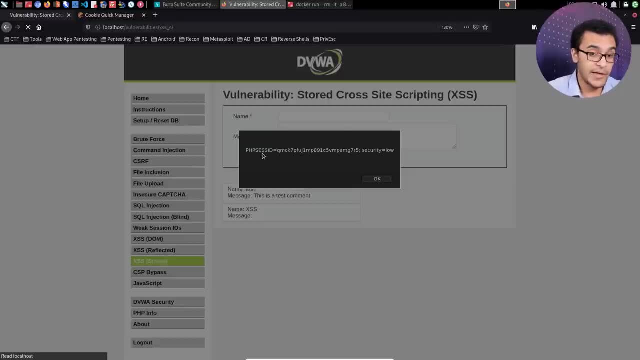 and then i'll say: sign guest book. all right, so you can see that when that attribute is disabled, when the http only attribute is disabled because i've been able to inject that cross-site, that javascript code onto this page, the javascript is executed and in this case, 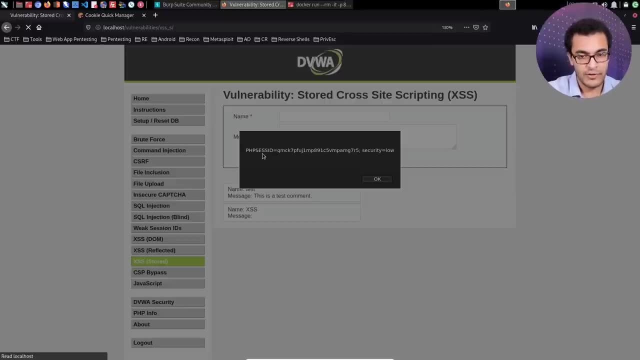 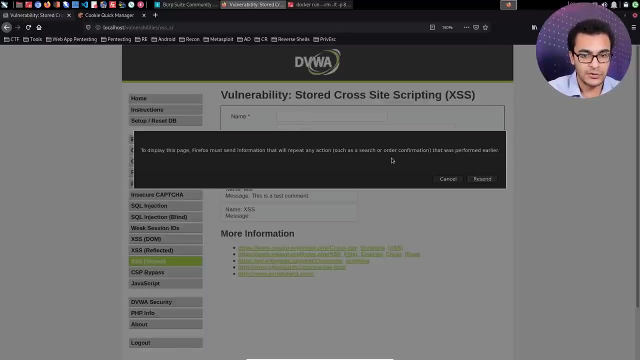 for the purpose of this example, the cookie of of a particular user, in this case myself, is displayed to me. but if you're aware of cross-site scripting, there's multiple ways uh, you can sort of uh get that information. so let's try it again, all right, so if i refresh it, just to show you. 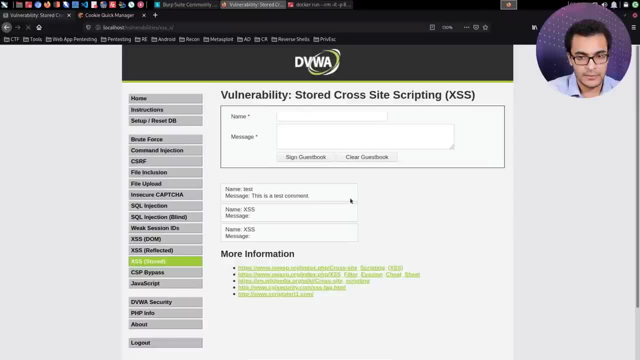 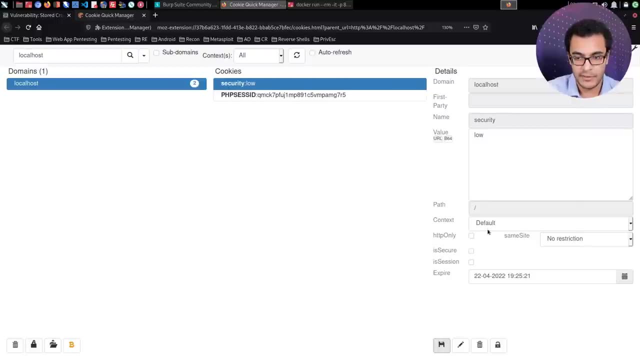 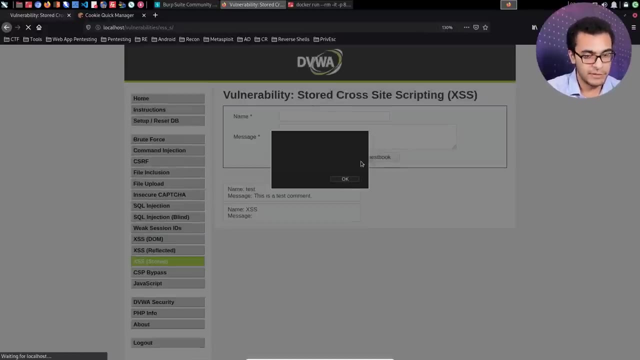 it's displayed again because it's being: uh okay, so it's working. so i think we actually resubmitted that. but this will work perfectly fine. so i'll just enable http only now. so http only there we are. if i refresh that send, you can now see, because we have enabled. 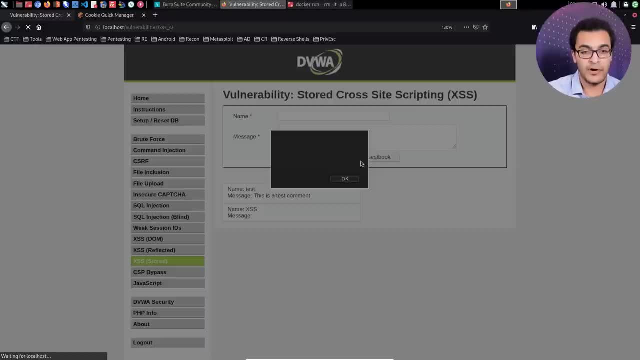 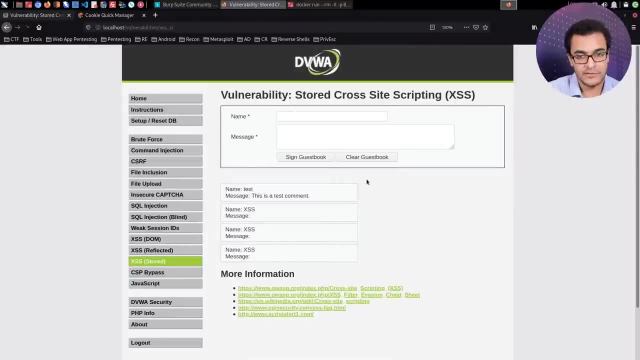 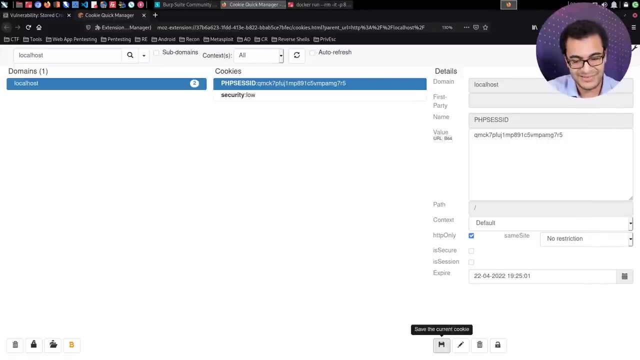 that attribute. uh, we cannot interact with the cookie via client-side javascript, so that information is essentially kept secure. you're starting to understand how important this is. now all right, so that was one of the examples. now, what i also wanted to cover again, and this is i'm not really sure whether i wanted to cover it, but uh, if we take a look at the is secure one. this: 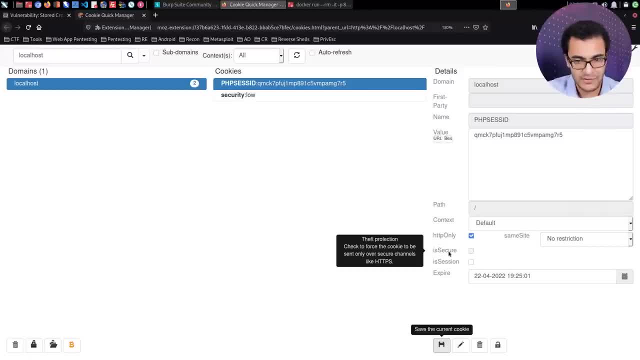 will only force this, will check to force the cookie to be sent over only over secure channels, but that's really not important. but we can actually check it out to see how it works. so you know, that works out just fine. and then of course we have the same site, uh, port. 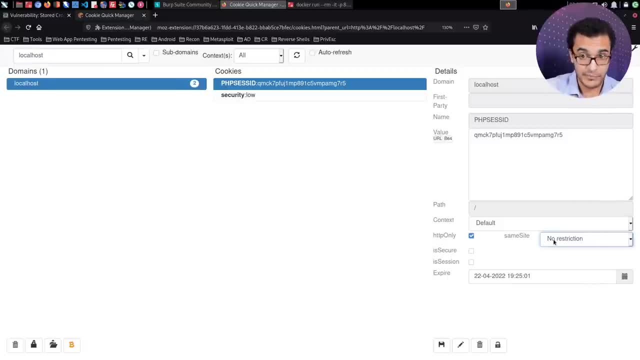 as well. now, since i've already done this, we're going to see that we've got access to our blocker again, so we'll just go ahead and do that and we're going to click on all right, so we've got the javascript node and then we're going to go over to the next step and there will 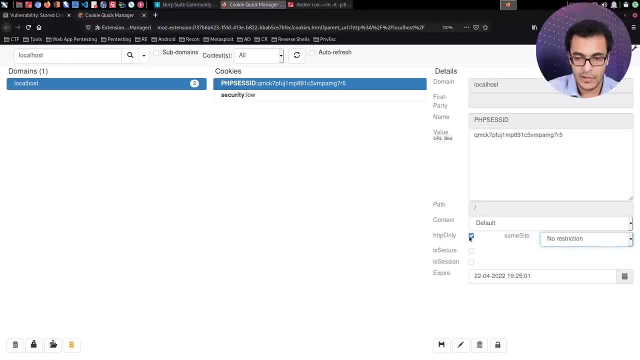 be a message in the status box showing the directory we want to edit and we're going to go back to the library so you can see that we've got the shared data file, the data query. there's also the data tool, which is what we've selected from the data point of view, but it allows. 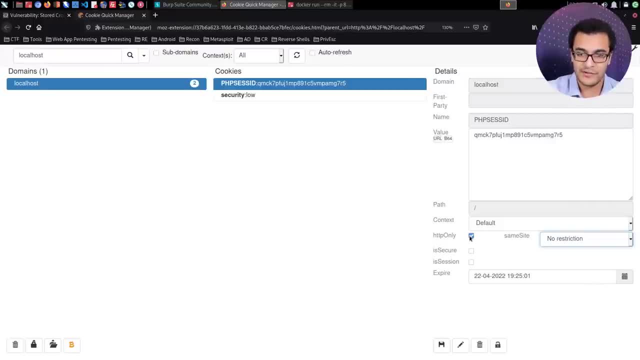 us to set up a set of parameters that are the default attributes, or what we do in our service, to set up a set of parameters or to set up a set of parameters. so in this case, i'm just going to set the default attributes. we can do that right now, so i'm going to go to the lets. 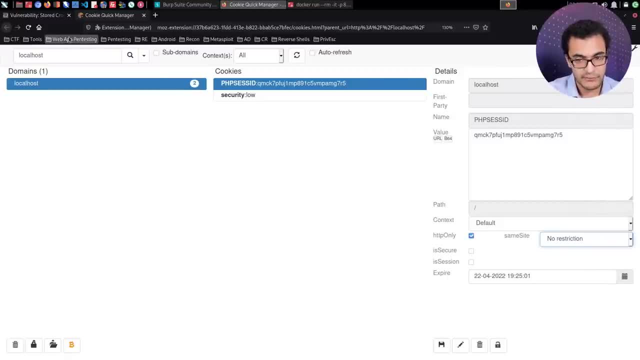 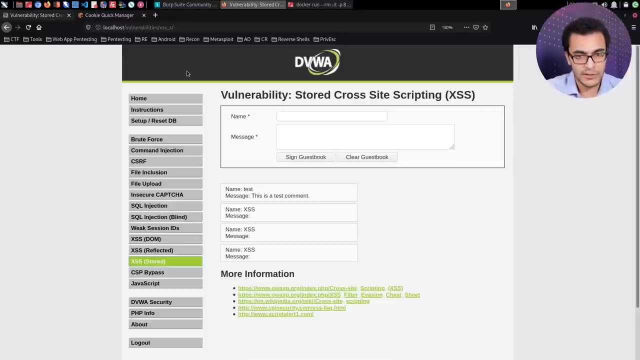 end. so that means that the, the actual server really, or the actual web developer himself, is really in control of cookie security, if you will. so the other way we can do this is we can actually test the security of cookies with birth suite. so let me just switch over there. so I'm just gonna say home. so 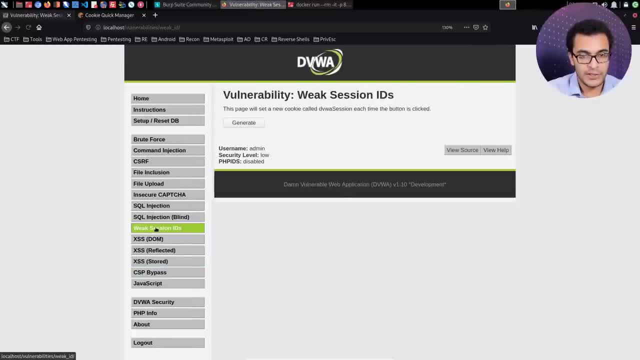 what I'll do here now is let's head over into week session IDs and we. what I want to do is let me just enable the intercept, so this page will set a new cookie called the damn vulnerable web app session each time the button is clicked. so just take note of that. I'll explain what this means so we can click. 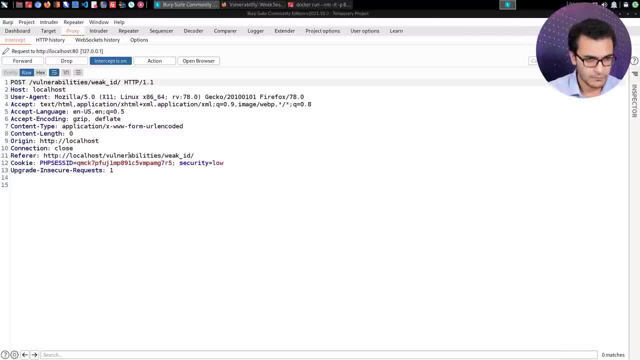 on generate and you can see now, in this case did it actually do it. let's say forward once again. we say generate again. there we are. so D the damn vulnerable web app session is now in the web app session. so let me just say forward once again. we say generate again. there we are. so D the damn vulnerable web app session ID. so this is. 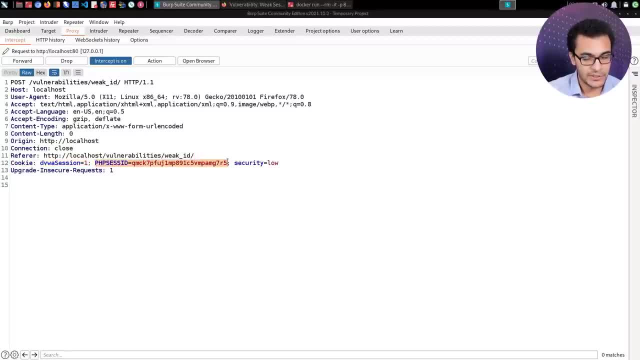 testing session IDs, so disregard PHP session ID for now. that's that's done by PHP itself, so just keep that in mind. what we are testing here is the security of a session ID. now this is weak. why is it weak? if you remember the slides, this is not random. it looks sequenced because it's starting from one. let's test it a. 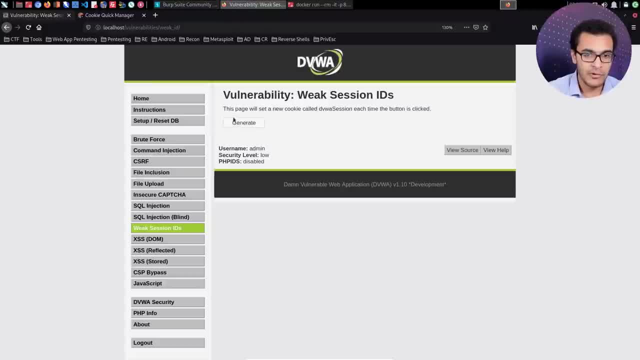 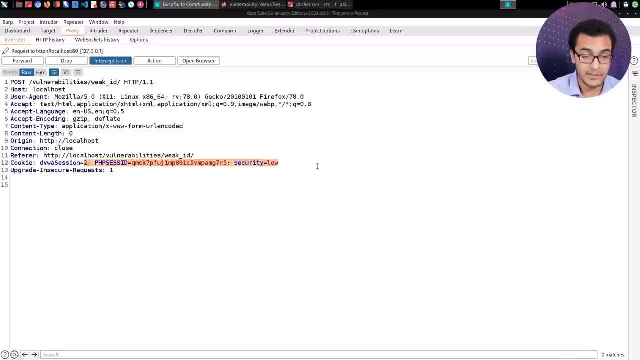 little bit more. hmm, I'll say forward. let's click on generate again. ah, so the next session IDs to all right. so from the perspective of an attacker, if they know that this is not random and it's sequentially handled, then they can just type in whatever number they want and they'll be able to sort of. 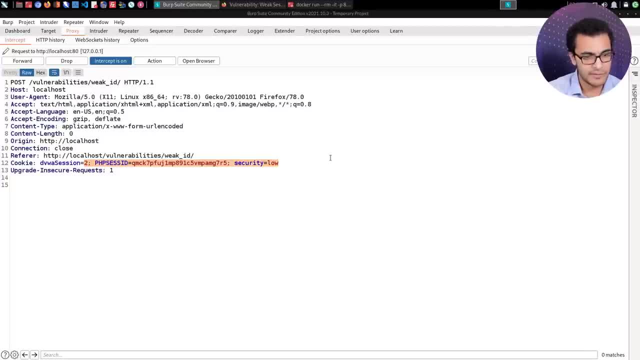 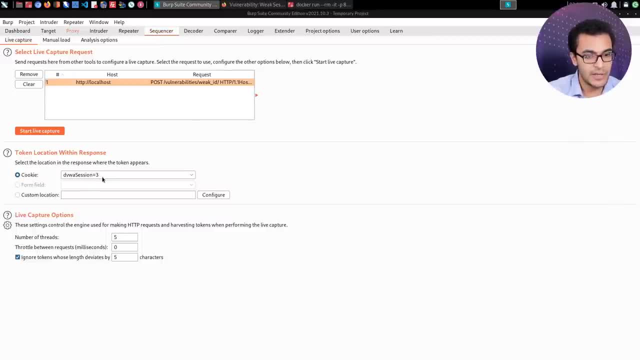 sequencer here. so I'll send that to the sequencer here. and we can you know sequencer here. so I'll send that to the sequencer here and we can you know specify the cookie? so dvwa, session 3, and specify the cookie? so dvwa, session 3. and. 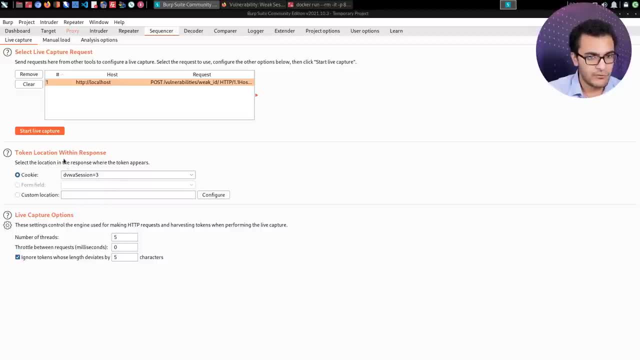 specify the cookie. so dvwa, session 3, and you know, let's see what do we need to. you know, let's see what do we need to. you know, let's see what do we need to modify anything here we can just start. modify anything here, we can just start. 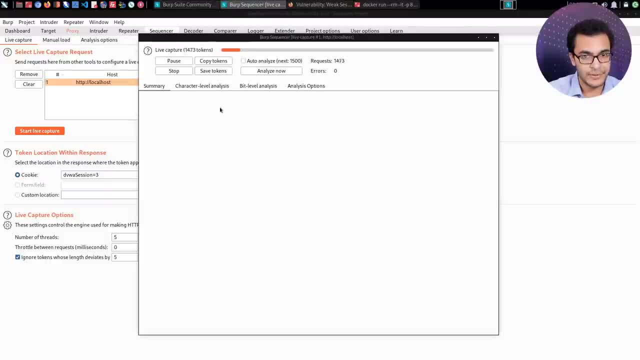 modify anything here. we can just start the live capture. so it's going to go the live capture. so it's going to go the live capture so it's going to go through. um, there we are, it's going to through. um, there we are, it's going to. 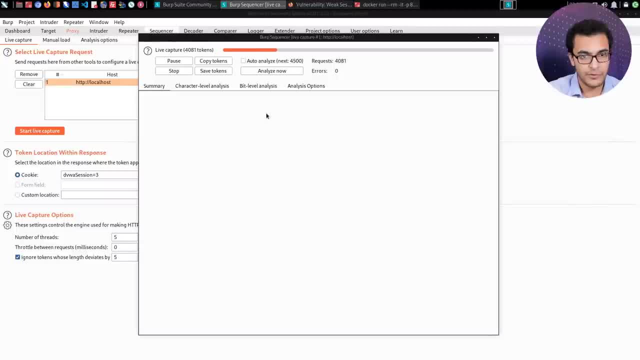 through um. there we are. it's going to begin the live capture. so it's going begin the live capture. so it's going begin the live capture. so it's going through all the the actual requests and through all the the actual requests and through all the the actual requests and tokens. so we'll give this as a couple of. 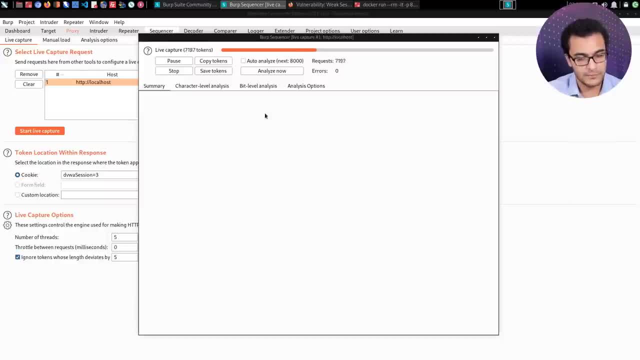 tokens. so we'll give this as a couple of tokens. so we'll give this as a couple of seconds to complete and I'll explain why seconds to complete and I'll explain why seconds to complete and I'll explain why we're using this. we're using this. 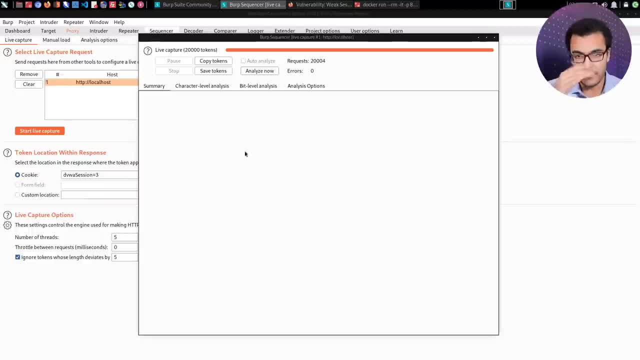 we're using this. so uh again, remember this is being done. so uh again, remember this is being done. so uh again, remember this is being done for the low security level, which is for the low security level, which is for the low security level, which is expected. that's what DVWA is. uh was. 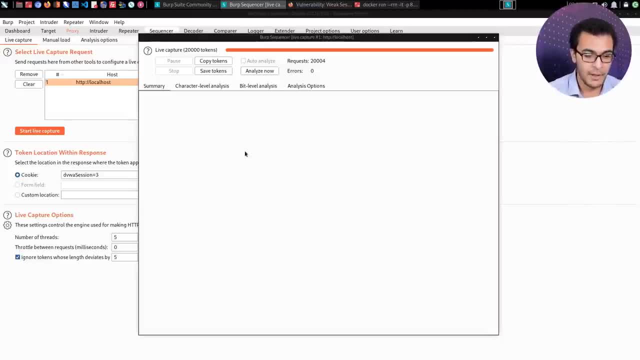 expected. that's what DVWA is uh was expected. that's what DVWA is uh was developed to do is to show you how developed to do is. to show you how developed to do is. to show you how security differs from poorly secured. security differs from poorly secured. 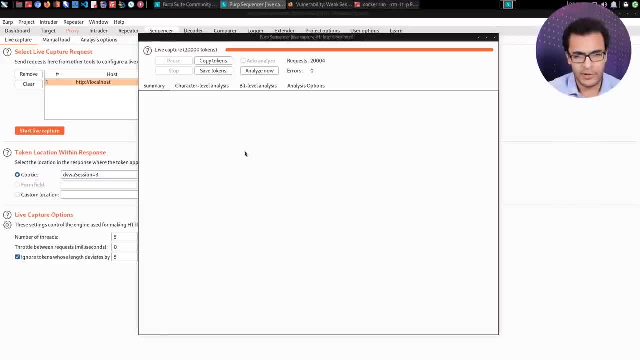 security differs from poorly secured sites to sites to sites to, I would say quite uh, quite well secured. I would say quite uh, quite well secured. I would say quite uh, quite well secured. site so we can click on analyze now. site so we can click on analyze now. 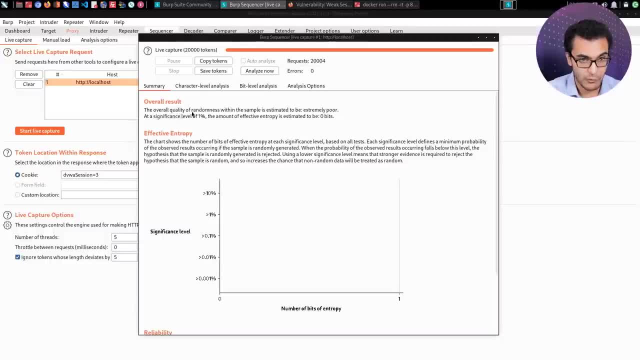 site so we can click on analyze now and you can see right over here the and you can see right over here the and you can see right over here the overall result, the overall quality of overall result. the overall quality of overall result, the overall quality of randomness within the sample is. 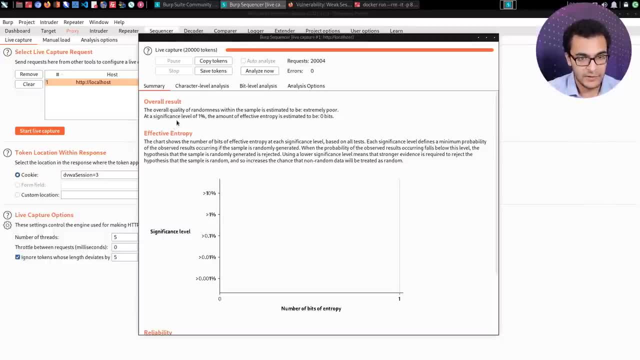 randomness within the sample is: randomness within the sample is estimated to be extremely poor. estimated to be extremely poor. estimated to be extremely poor at a significance level of one percent. at a significance level of one percent. at a significance level of one percent, the amount of effective entropy is: 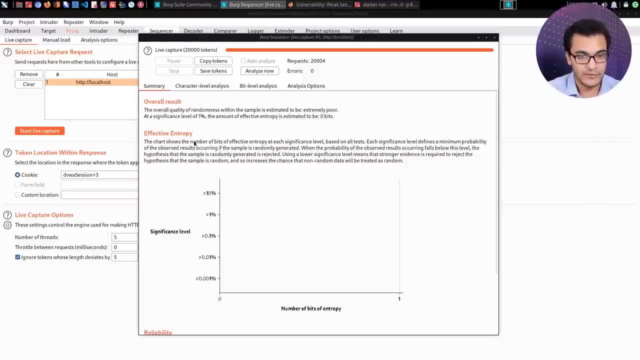 the amount of effective entropy is the amount of effective entropy is estimated to be zero bits. estimated to be zero bits. estimated to be zero bits. so effective entropy: the chart shows the so effective entropy. the chart shows the so effective entropy. the chart shows the number of bits of effective entropy at. 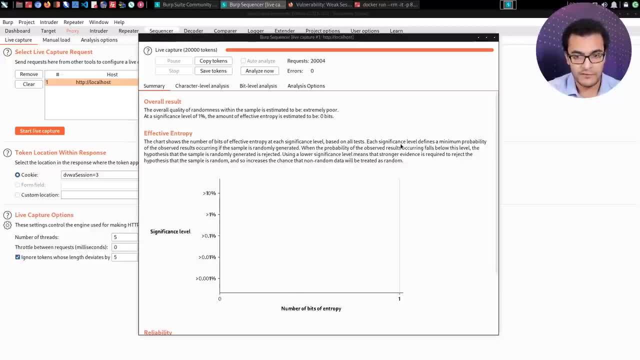 number of bits of effective entropy. at number of bits of effective entropy at each significance level, based on all each significance level, based on all. each significance level, based on all tests. each significance level defines a tests. each significance level defines a tests. each significance level defines a minimum probability of the observed. 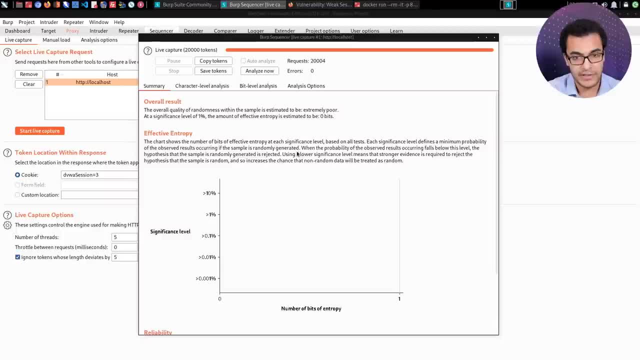 minimum probability of the observed. minimum probability of the observed results occurring in. results occurring in. results occurring in. if the sample is randomly generated when. if the sample is randomly generated when: if the sample is randomly generated when, the probability of the observed results. the probability of the observed results. 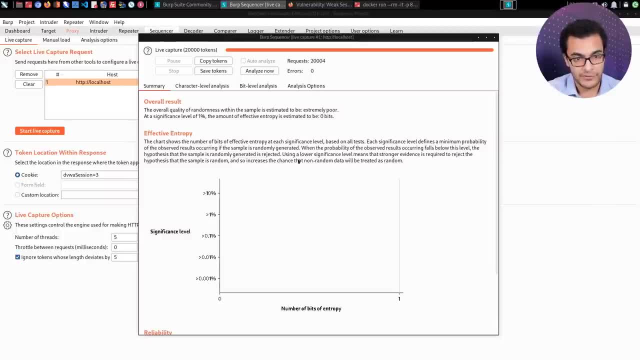 the probability of the observed results occurring falls occurring falls. occurring falls below this level. the hypothesis below this level, the hypothesis below this level, the hypothesis that the sample is randomly generated, that the sample is randomly generated, that the sample is randomly generated, is rejected using a lower significance. 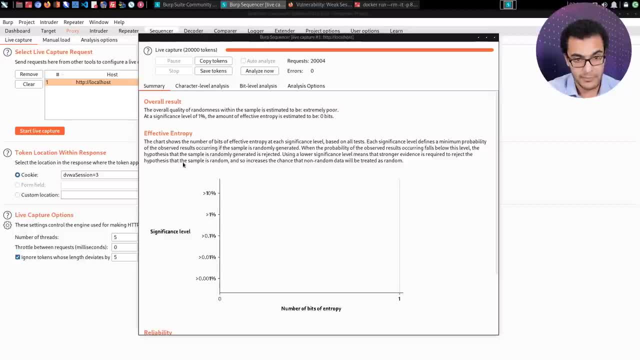 is rejected using a lower significance is rejected using a lower significance. level means level means level means that strong evidence is required to that strong evidence is required to that strong evidence is required to reject the hypothesis that the sample is, reject the hypothesis that the sample is, reject the hypothesis that the sample is random and so increases the chance. 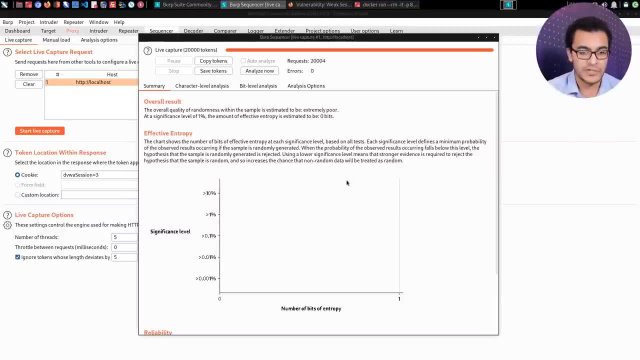 random, and so increases the chance random, and so increases the chance that non-random data will be treated as that. non-random data will be treated as that. non-random data will be treated as random. so this essentially tells you: uh, random. so this essentially tells you: uh, random. so this essentially tells you: uh, you know. 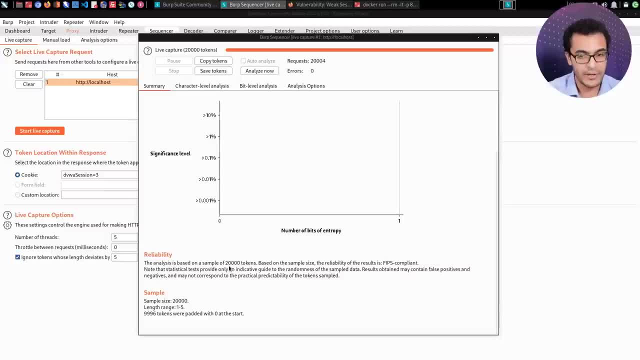 you know. you know, if you scroll down right over here, you, if you scroll down right over here, you, if you scroll down right over here, you know, the it'll actually give you a know. the it'll actually give you a know. the it'll actually give you a more information regarding this particular. 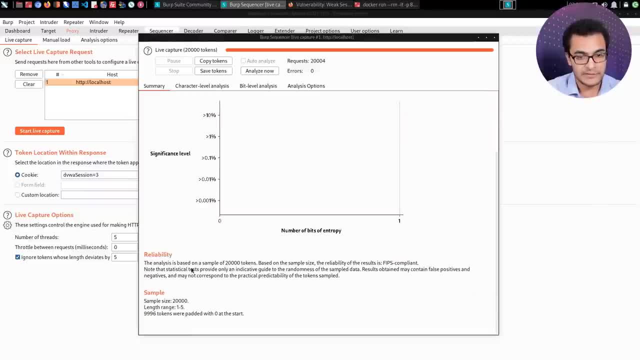 more information regarding this particular, more information regarding this particular live capture and analysis. live capture and analysis. live capture and analysis. but it's essentially telling us that, um, but it's essentially telling us that, um, but it's essentially telling us that, um, that this is, uh, this, extremely poor. 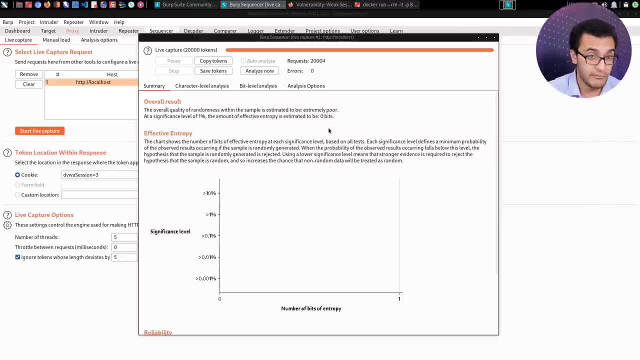 that this is, uh this extremely poor, that this is, uh this extremely poor. because it seems to be, uh, there doesn't. because it seems to be, uh, there doesn't. because it seems to be, uh, there doesn't seem to me to be any randomness involved, seem to me to be any randomness involved. 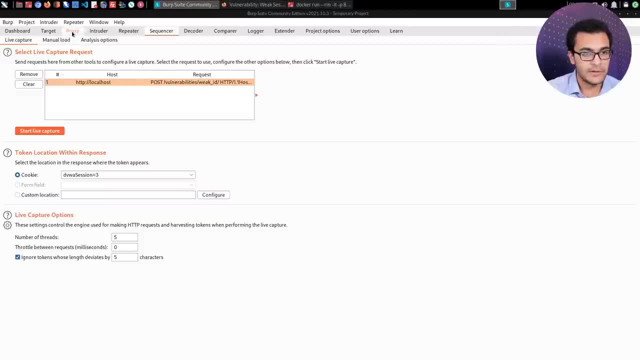 seem to me to be any randomness involved. so, um, what i'll do now. so, um, what i'll do now. so, um, what i'll do now is: uh, we'll go back to the proxy let's is: uh, we'll go back to the proxy let's. 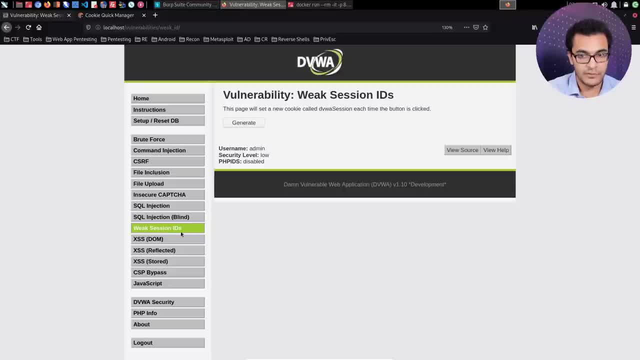 is: uh, we'll go back to the proxy. let's forward that there. let me just disable forward that there. let me just disable forward that there. let me just disable intercept for a second. uh, we'll set this intercept for a second. uh, we'll set this intercept for a second. uh, we'll set this to high so. 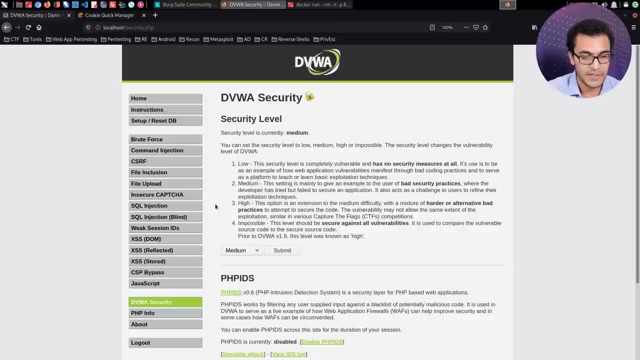 to high. so to high. so dvwa security: we'll actually set it to dvwa security. we'll actually set it to dvwa security. we'll actually set it to medium, and we'll test that out as well. medium, and we'll test that out as well. 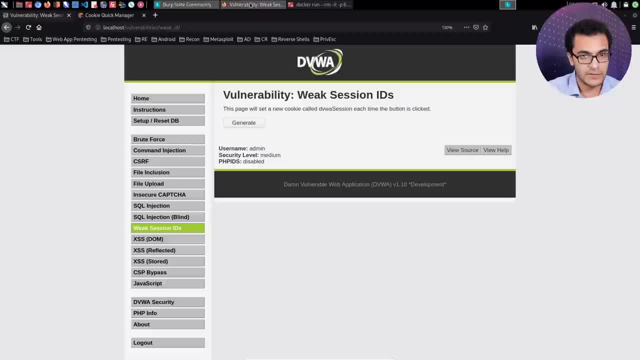 medium, and we'll test that out as well. uh, weak session ids- uh, let me make sure, uh, weak session ids- uh, let me make sure, uh, weak session ids- uh, let me make sure. intercept is on. intercept is on. intercept is on generate. okay, so we now have something a. 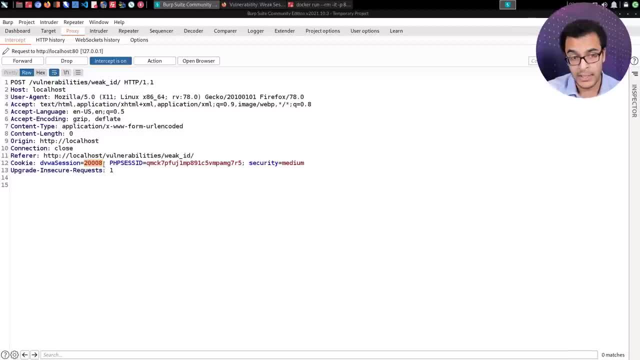 generate okay. so we now have something a generate okay. so we now have something a little bit more complex. doesn't really little bit more complex? doesn't really little bit more complex? doesn't really look random, it could be. look random, it could be. look random, it could be. but it's quite short. that could be a. 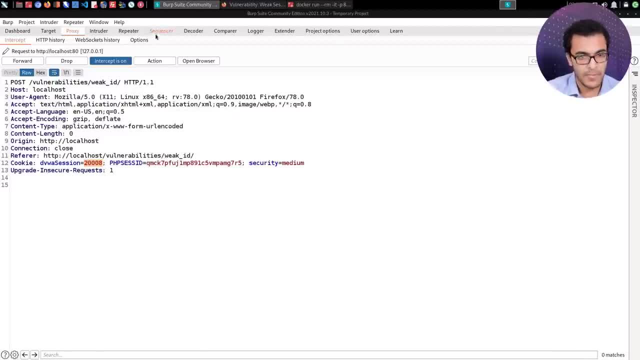 but it's quite short. that could be a, but it's quite short. that could be a potential issue, right? so let's send this potential issue right. so let's send this potential issue right. so let's send this to the sequencer again, to the sequencer again. 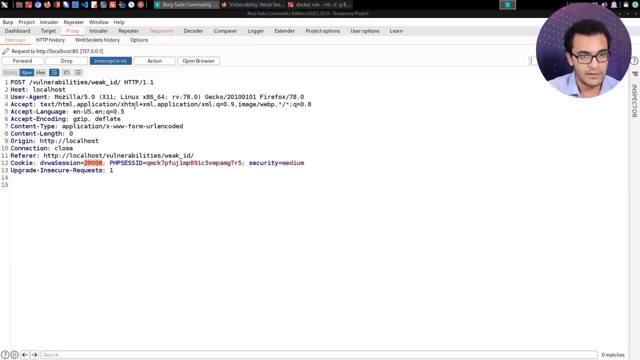 to the sequencer again. all right sequencer. uh, let me just get all right sequencer. uh, let me just get all right sequencer. uh, let me just get rid of that there and i'll send it again. rid of that there, and i'll send it again. 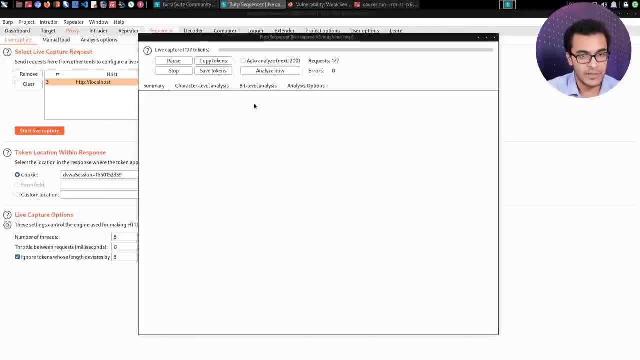 rid of that there and i'll send it again. should have done that previously, but should have done that previously, but should have done that previously. but there we go um and we'll start the live. there we go um and we'll start the live. there we go um and we'll start the live capture. so again, just gonna wait for. 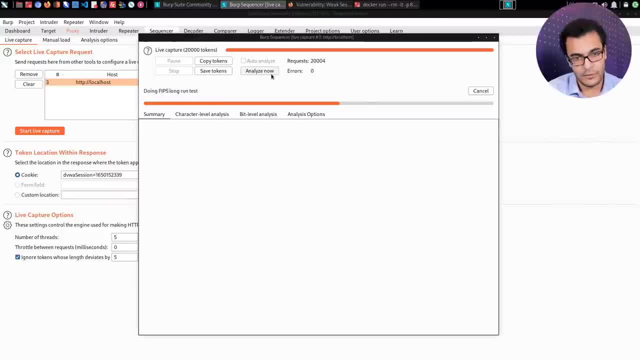 capture. so, again, just gonna wait for capture. so again, just gonna wait for this to complete this, to complete this, to complete. all right, so let's analyze the medium. all right, so let's analyze the medium. all right, so let's analyze the medium security level. so, security level. so let's analyze the medium security level. so, in this case, it looks like 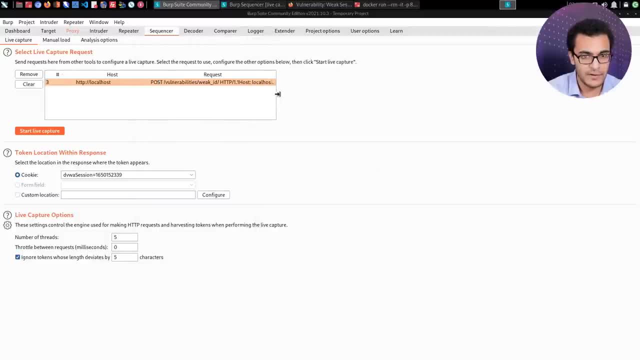 in this case it looks like. in this case it looks like it's the same here. i'm not really sure it's the same here. i'm not really sure it's the same here. i'm not really sure whether that is, whether that is, whether that is. uh, yeah, that's the correct request there. 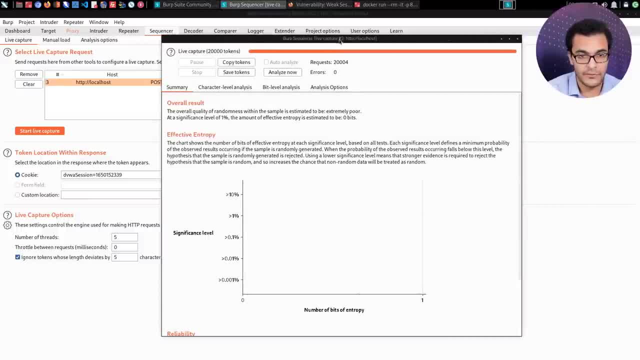 uh, yeah, that's the correct request there. uh, yeah, that's the correct request there. but you know it's still telling us that. but you know it's still telling us that, but you know it's still telling us that it the security here, the randomness uh. it the security here, the randomness uh. 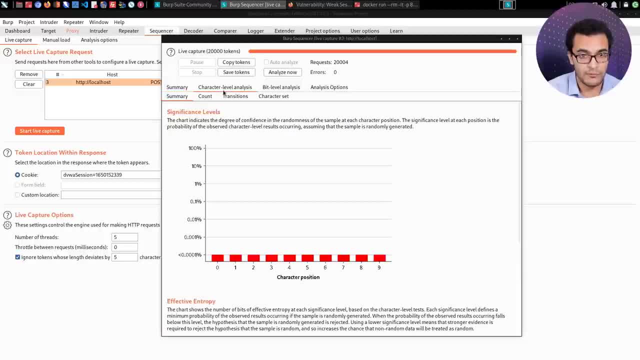 it, the security here, the randomness- uh is, uh is, uh is uh, extremely poor. so if we take a look at extremely poor, so if we take a look at extremely poor, so if we take a look at the actual um, no, i think this is still the actual um. no, i think this is still. 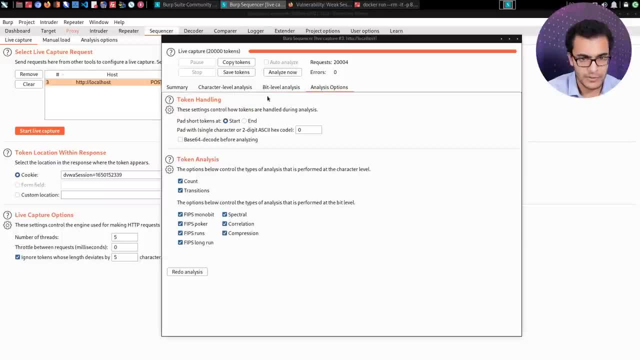 the actual. um. no, i think this is still character position. character position, character position, bit position. yeah, i think that's the bit position. yeah, i think that's the bit position. yeah, i think that's the correct one, but um correct one, but um. correct one, but um, if we go back, 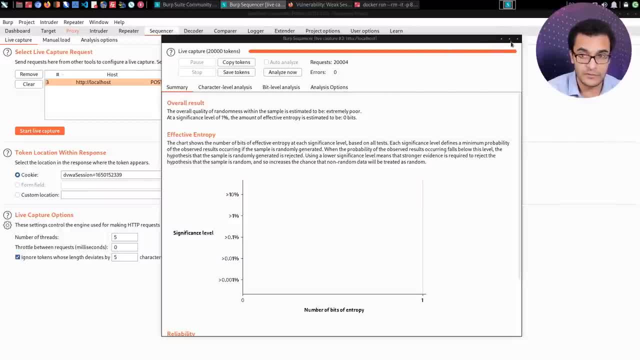 if we go back, if we go back here, all right right. oh yeah, that that's here. all right right. oh yeah, that that's here. all right right. oh yeah, that that's the correct one. so again, it's still poor. the correct one. so again, it's still poor. 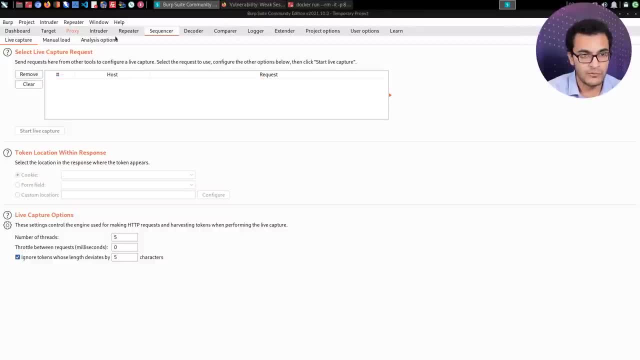 the correct one. so again, it's still poor. so let's just repeat the process once. so let's just repeat the process once. so let's just repeat the process once more, more, more. so remove and we'll go to proxy for. so remove and we'll go to proxy for. 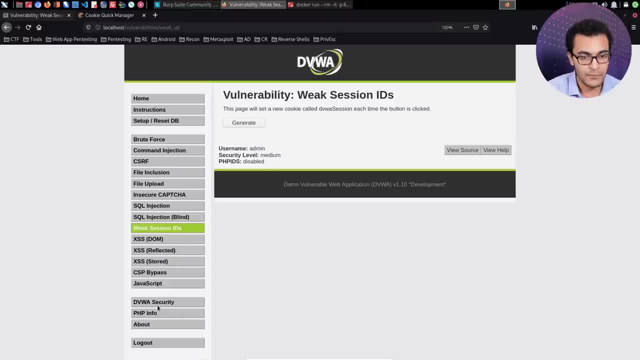 so remove and we'll go to proxy for that that. let me just disable intercept here. let me just disable intercept here. let me just disable intercept here. dvwa security: let's set it to high. dvwa security: let's set it to high. dvwa security: let's set it to high. maybe we'll get a better level here. 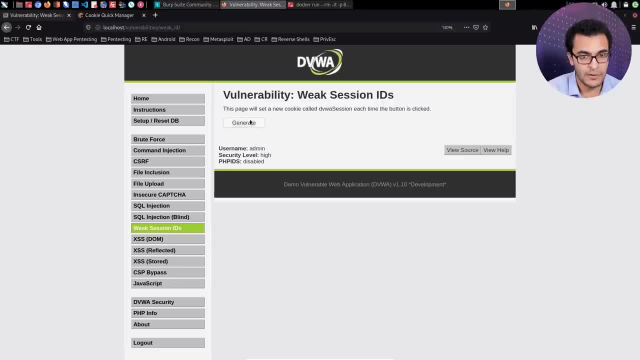 maybe we'll get a better level here. maybe we'll get a better level here. weak session ids. weak session ids. weak session ids. intercept on intercept on intercept on: generate- okay, that looks much better now. generate- okay, that looks much better now. generate- okay, that looks much better now, so we can send this to the sequencer. 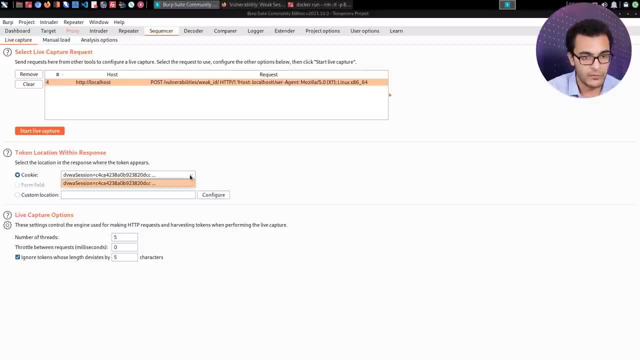 so we can send this to the sequencer. so we can send this to the sequencer. there we go um. let's make sure that is there. we go um. let's make sure that is there. we go um. let's make sure that is correct. it looks like it is. 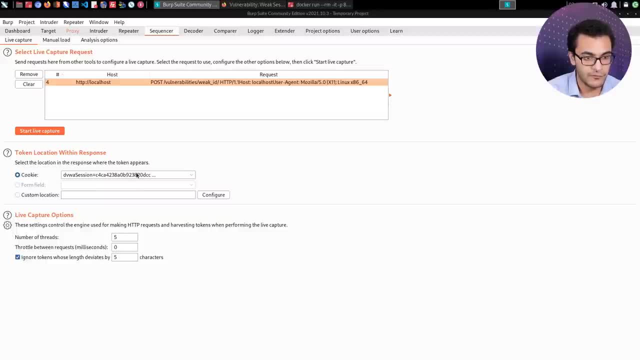 correct. it looks like it is correct. it looks like it is. that's the cookie there. uh, it's not that's the cookie there. uh, it's not. that's the cookie there. uh, it's not from a form field or a custom location. from a form field or a custom location. 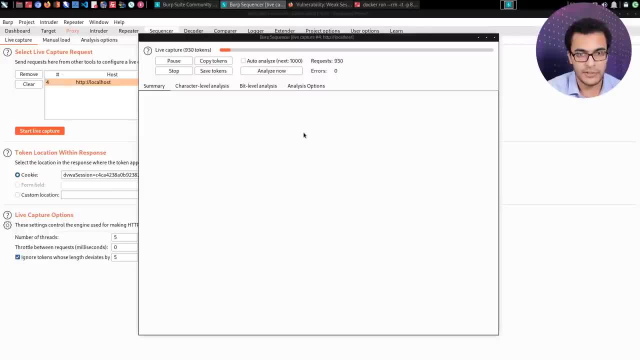 from a form, field or a custom location. so that's the actual token. so let's, so. that's the actual token, so let's, so. that's the actual token. so let's start that here. it should only take a start that here. it should only take a. 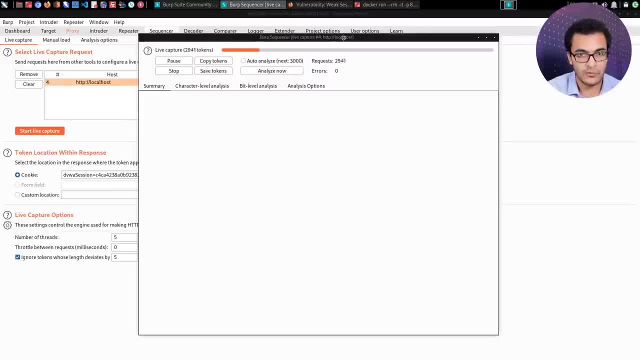 start that here. it should only take a couple of seconds. couple of seconds, couple of seconds. hopefully i don't have to, um, hopefully i don't have to, um, hopefully i don't have to, um, i don't actually have to uh wait for this. i don't actually have to uh, wait for this. 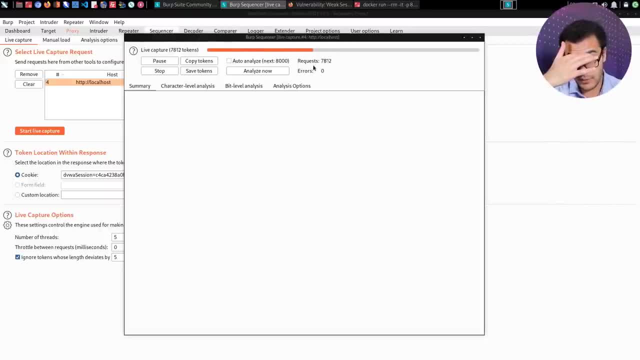 i don't actually have to uh, wait for this to complete, but this you can actually to complete, but this you can actually to complete, but this you can actually see. it seems to be a high level of see. it seems to be a high level of see. it seems to be a high level of entropy in this case, because it's taking 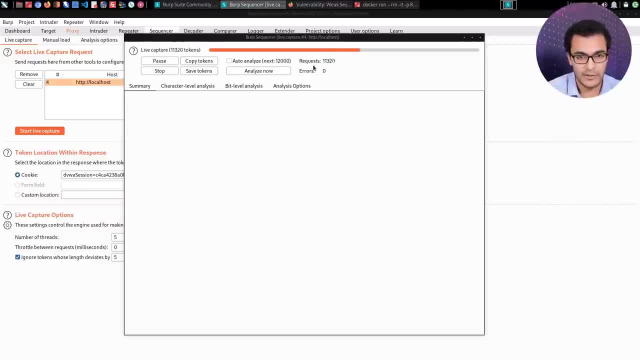 entropy in this case because it's taking entropy, in this case because it's taking much longer. but we'll actually see what much longer, but we'll actually see what much longer, but we'll actually see what the summary is. the summary is. the summary is so: um, just gonna wait for this to 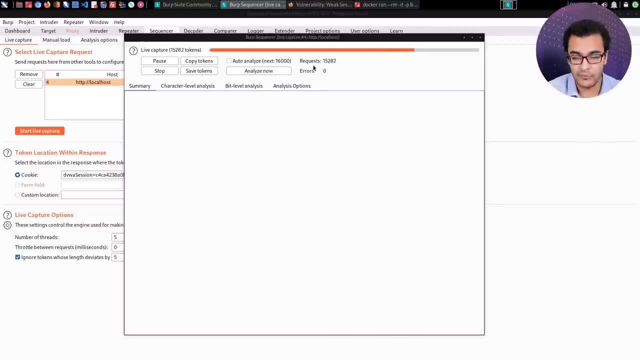 so, um, just gonna wait for this to so, um, just gonna wait for this to complete and we should be able to wrap complete, and we should be able to wrap complete and we should be able to wrap up this video then and move on to up this video then and move on to. 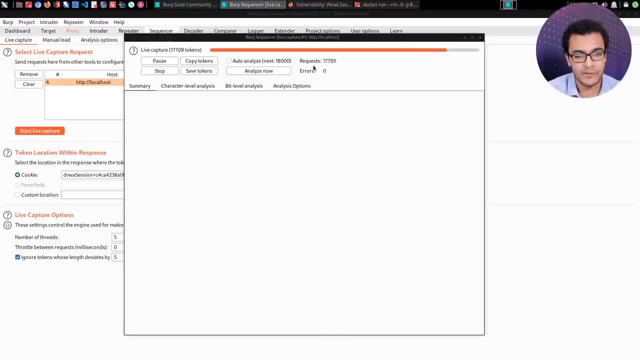 up this video then and move on to the next video where we'll be covering how, the next video where we'll be covering how, the next video where we'll be covering how to use burp suite. because to use burp suite? because to use burp suite? because, uh, you know, if you're not familiar with. 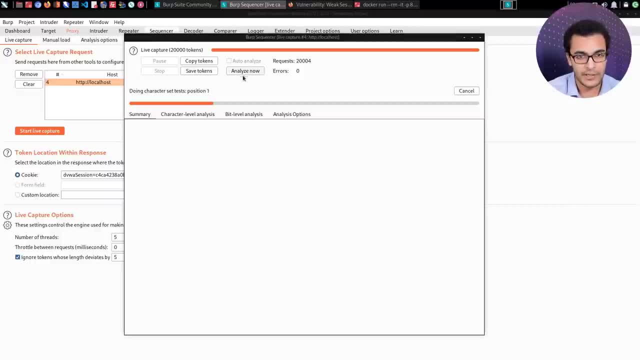 uh, you know, if you're not familiar with, uh, you know, if you're not familiar with burp suite, then you know you're half as burp suite, then you know you're half as burp suite, then you know you're half as effective. so analyze now. 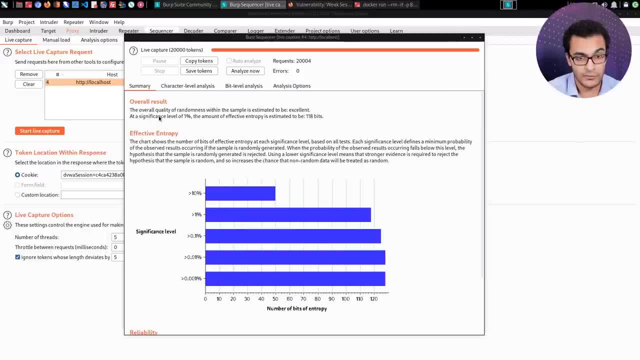 all right, taking a bit there, we are all right. taking a bit there. we are all right taking a bit there. we are fantastic. so the overall quality of fantastic, so the overall quality of fantastic, so the overall quality of randomness within the sample is. randomness within the sample is. 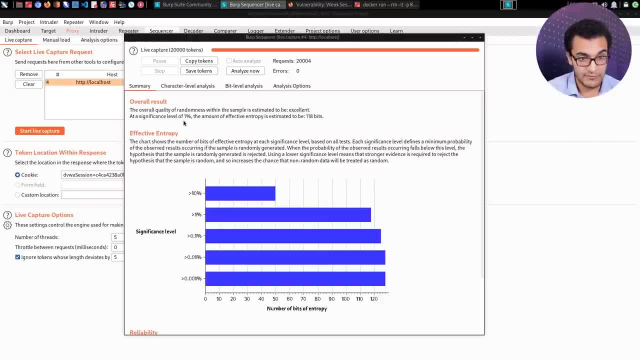 randomness within the sample is estimated to be excellent. estimated to be excellent. estimated to be excellent at a significance level of one percent. at a significance level of one percent. at a significance level of one percent, the amount of effective entropy is the amount of effective entropy is. the amount of effective entropy is estimated to be 118 bits. you can take a. 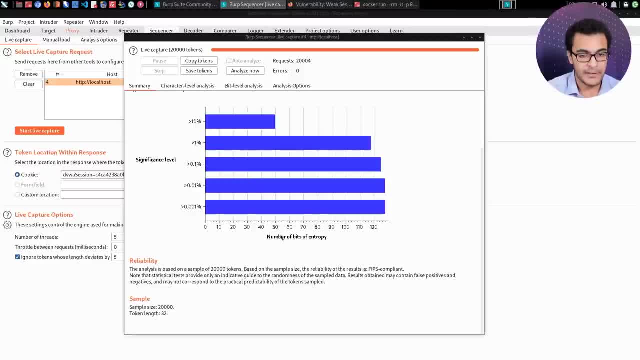 estimated to be 118 bits. you can take a estimated to be 118 bits. you can take a look at this, look at this, look at this: the significance level there and the. the significance level there and the. the significance level there and the reliability right. so it'll tell you what. 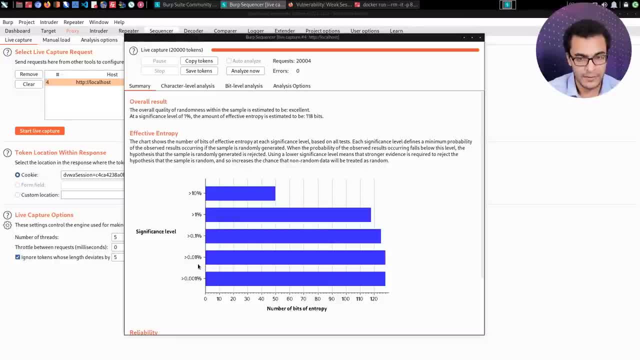 reliability. right, so it'll tell you what reliability. right, so it'll tell you what sample size it used and the token sample size it used and the token sample size it used and the token length. so again the the most important length. so again, the the most important. 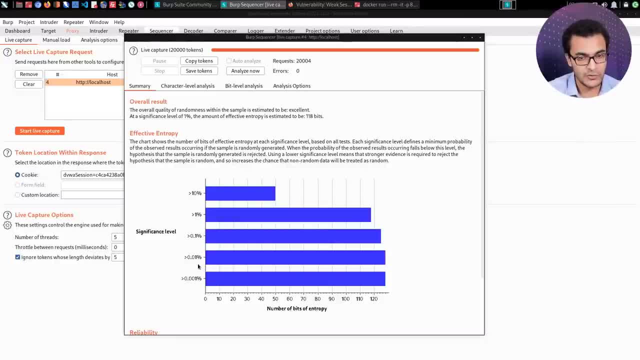 length. so again, the the most important thing is the actual length thing, is the actual length thing, is the actual length of the, the actual token itself, or the of the, the actual token itself, or the of the, the actual token itself, or the session id, if you will. uh and uh, the. 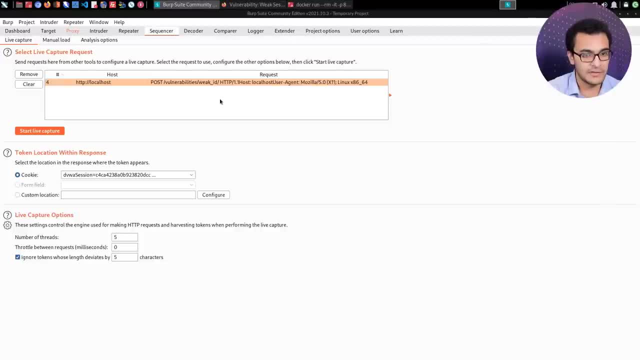 session id. if you will uh and uh the session id, if you will uh and uh the actual randomness of it. so that's how actual randomness of it. so that's how actual randomness of it. so that's how you can analyze a session id um security. you can analyze a session id um security. 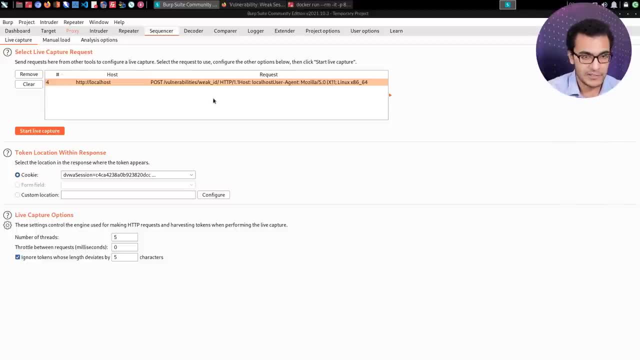 you can analyze a session id um security if you will, and of course this ties into if you will, and of course this ties into if you will. and of course this ties into bug bounty. so maybe that's a little tip. bug bounty, so maybe that's a little tip. 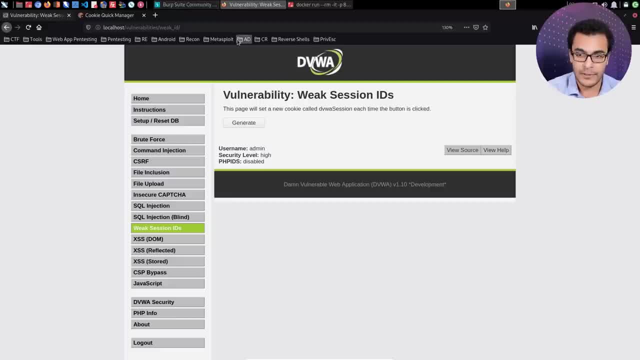 bug bounty. so maybe that's a little tip or trick for you guys there. so let's or trick for you guys there. so let's or trick for you guys there. so let's forward this here, um, we have set it to. forward this here, um, we have set it to. 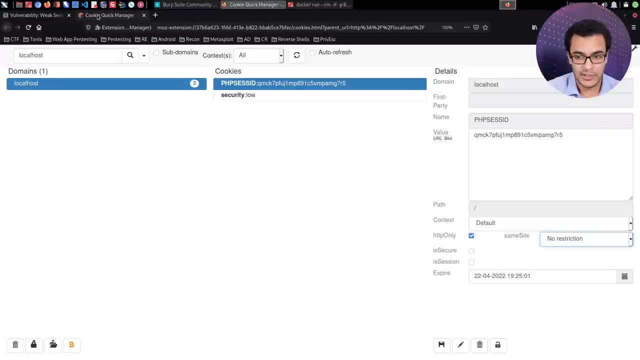 forward this here: um, we have set it to high now. i wonder whether the cookies high now. i wonder whether the cookies high now. i wonder whether the cookies have changed. i wonder, wonder, wonder have changed? i wonder, wonder, wonder have changed. i wonder, wonder, wonder. let's uh see, uh, we probably need to. 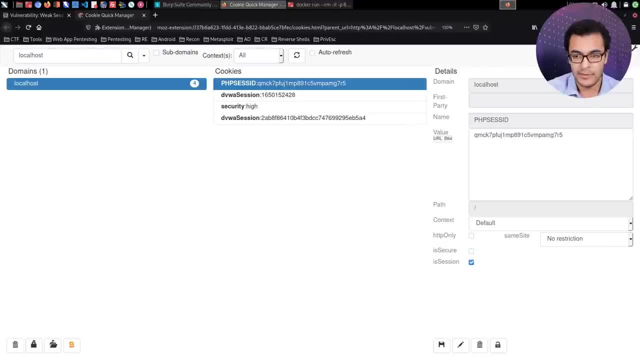 let's uh see, uh, we probably need to. let's uh see, uh, we probably need to re-authenticate, but uh, yeah, it's the re-authenticate. but uh, yeah, it's the re-authenticate. but uh, yeah, it's the same one here, same one here. 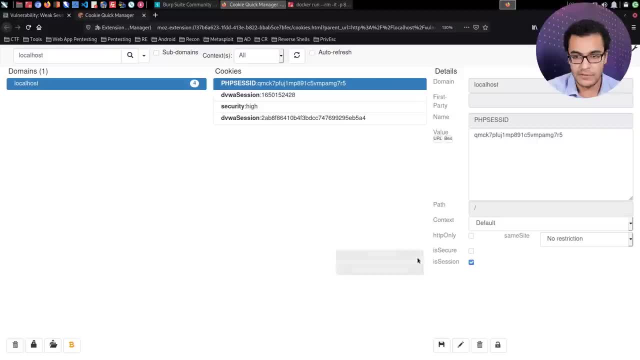 same one here. uh, the only difference as you can see, uh, the only difference as you can see, uh, the only difference as you can see. session: the the session is session session. the the session is session session. the the session is session. attribute is: uh, essentially. attribute is: uh, essentially. 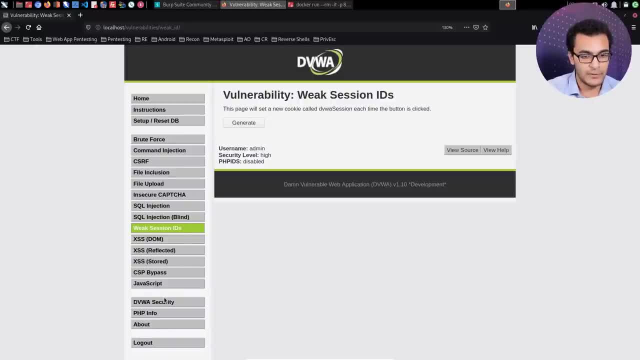 attribute is uh. essentially: uh checked or enabled um. uh checked or enabled. um. uh checked or enabled um. if we take a look at uh, let's see uh. if we take a look at uh, let's see uh. if we take a look at uh, let's see uh. i think we've gone through all the. 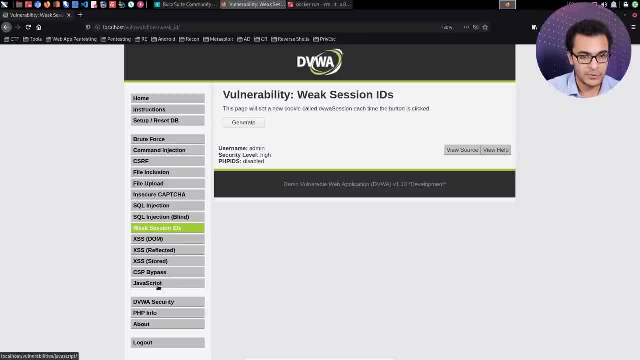 i think we've gone through all the. i think we've gone through all the examples that i wanted to highlight, examples that i wanted to highlight, examples that i wanted to highlight: uh, we pretty much only wanted to take a. uh, we pretty much only wanted to take a. 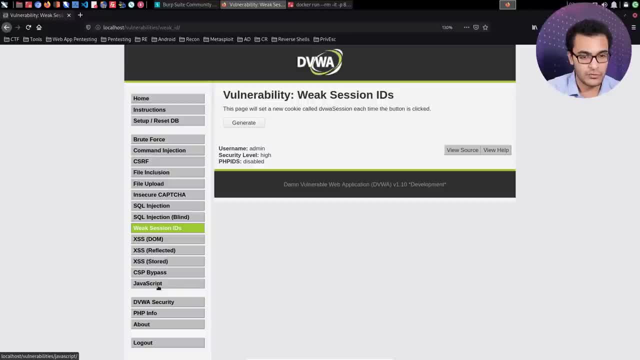 uh, we pretty much only wanted to take a look at session ids cookies and of look at session ids cookies and of look at session ids cookies and, of course, how that ties into cross-site course, how that ties into cross-site course, how that ties into cross-site scripting, which we have. 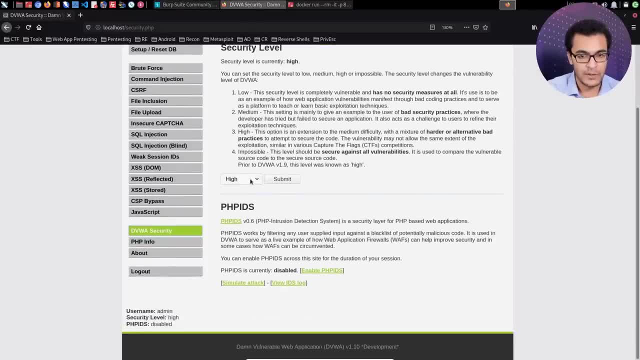 scripting which we have, scripting which we have- uh, let me just turn off intercept here. uh, let me just turn off intercept here. uh, let me just turn off intercept here. and of course you can continue testing and of course you can continue testing and of course you can continue testing with higher security levels. but yeah, i 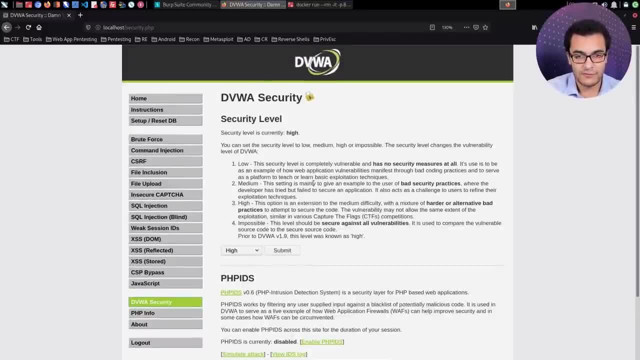 with higher security levels, but, yeah, i with higher security levels, but yeah, i think that's pretty much all that. i think that's pretty much all that. i think that's pretty much all that i wanted, wanted, wanted to cover in this video. let me know if to cover in this video. let me know if. 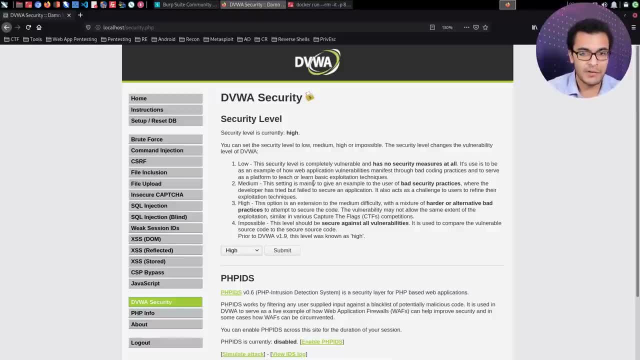 to cover in this video. let me know if you have any questions, or you know you have any questions, or you know you have any questions or you know suggestions. you can leave them in the suggestions. you can leave them in the suggestions. you can leave them in the comments section. if you want to contact. 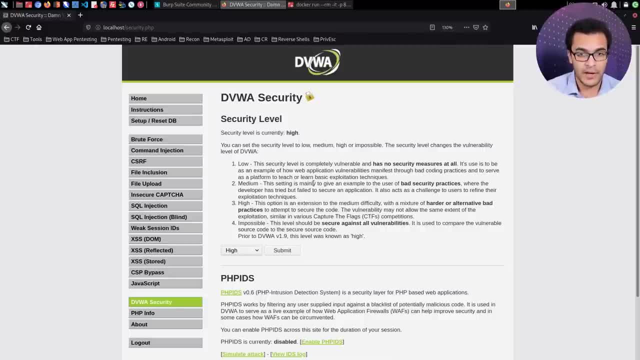 comments section. if you want to contact comments section. if you want to contact me directly, you can do so via twitter me directly. you can do so via twitter me directly. you can do so via twitter. or the actual hackers plate forum, the, or the actual hackers plate forum, the. 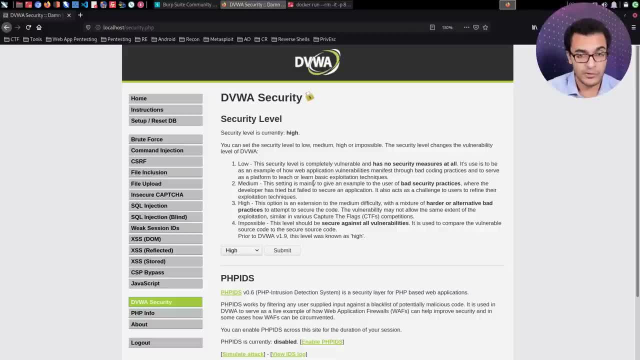 or the actual hackers plate forum. the link will be in the description and if link will be in the description and if link will be in the description and if you want to support the channel, you can. you want to support the channel, you can. you want to support the channel? you can do that via patreon. the link to that is: do that via patreon. the link to that is: do that via patreon. the link to that is also in the description section, with also in the description section, with also in the description section. with that being said, thank you very much for that being said. thank you very much for. 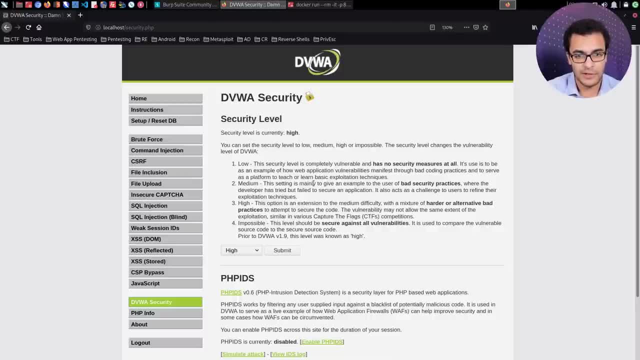 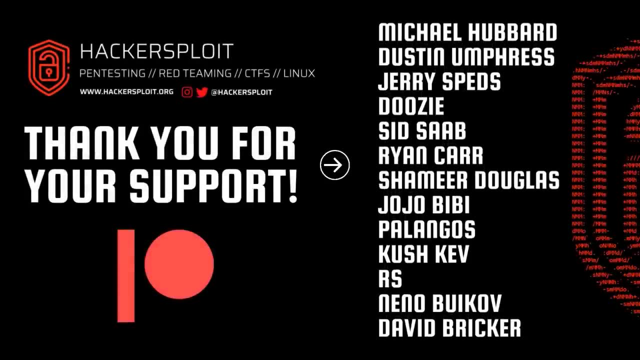 that being said, thank you very much for watching, watching, watching, and i'll be seeing you in the next and i'll be seeing you in the next and i'll be seeing you in the next video. i just want to take a couple of moments. i just want to take a couple of moments. 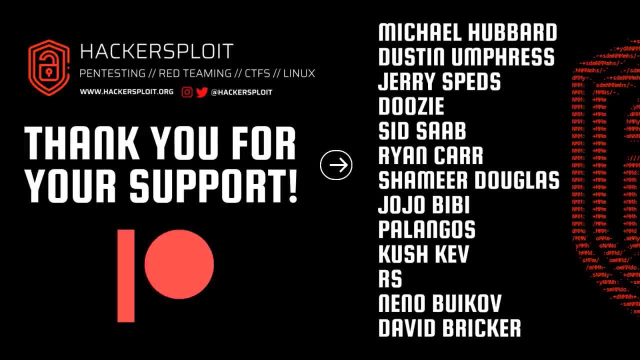 i just want to take a couple of moments: your bb balangos, kushkev rs, nino buikov, your bb balangos, kushkev rs, nino buikov, your bb balangos, kushkev rs, nino buikov and david bricker. you guys are really 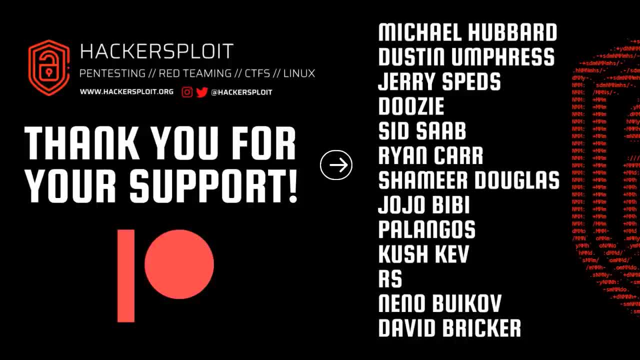 and david bricker, you guys are really- and david bricker, you guys are really awesome. thank you very much for awesome. thank you very much for awesome. thank you very much for supporting us and you guys make these supporting us and you guys make these supporting us and you guys make these types of videos possible, so we really 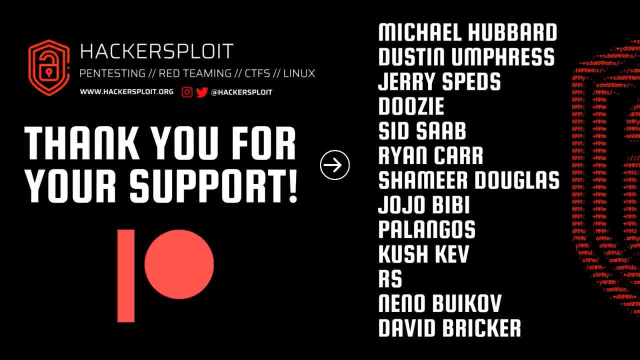 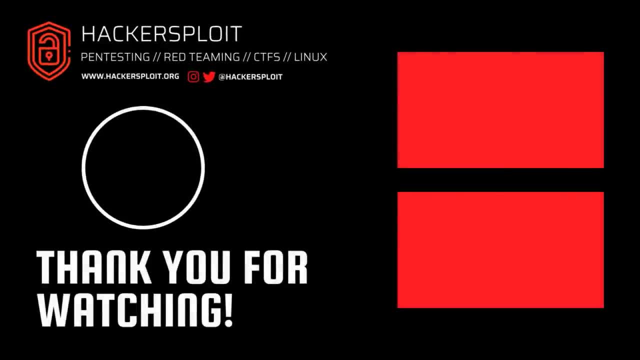 types of videos possible. so we really types of videos possible. so we really appreciate it and we look forward to appreciate it and we look forward to appreciate it and we look forward to producing even more high quality, producing even more high quality, producing even more high quality content.